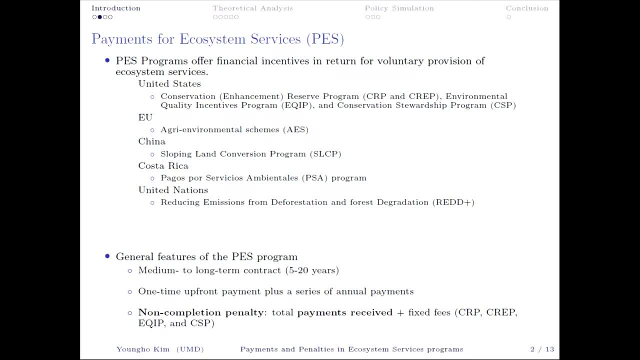 There's a non-completion penalty aspect feature which is the focus of our study. Because the contract is pretty long. there's a chance that farmers want to terminate the contract before expiration date. For example, in a CRP farmers convert their highly erodible crop land to grass cover, let's say During the 10-year. 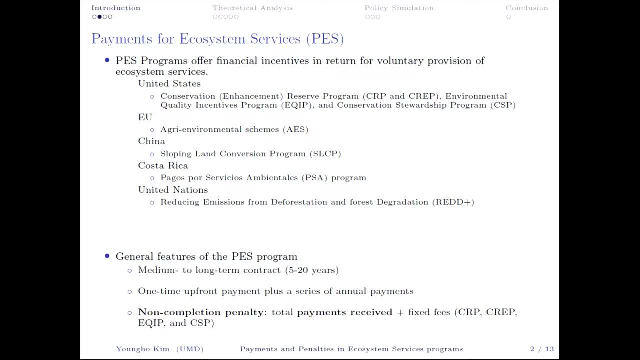 period contract. they might want to terminate the contract and produce crop. instead They want to get rid of the grass cover and produce crop again. Then in that case government want them to pay back penalty, all the termination penalty, The existing standard penalty structure in the 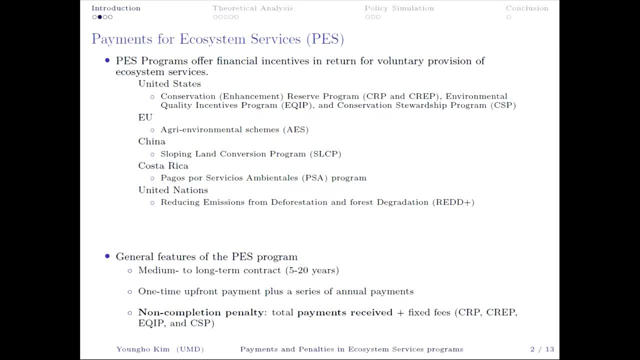 conservation policy is that government requires participants to pay back all payments, total payments, they have received so far. This penalty is an interesting policy instrument because it reduces contract all the termination but at the same time it affects participation incentives as well, Because if you're a farmer that has non-zero-termination 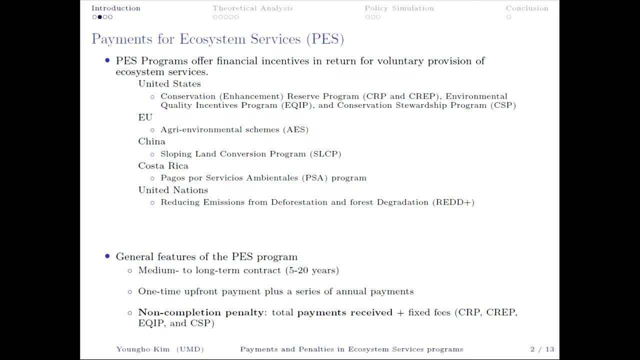 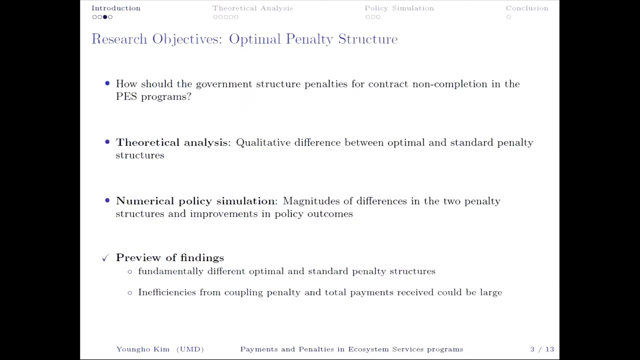 a zero chance of contract. all the termination during the contract period, then having high penalty in the offer contract will disincentivize eligible farmers to initially enroll in the program. Our research objective is to examine optimal penalty structure in the PES program. We conduct theoretical analysis to derive optimal penalty structure. 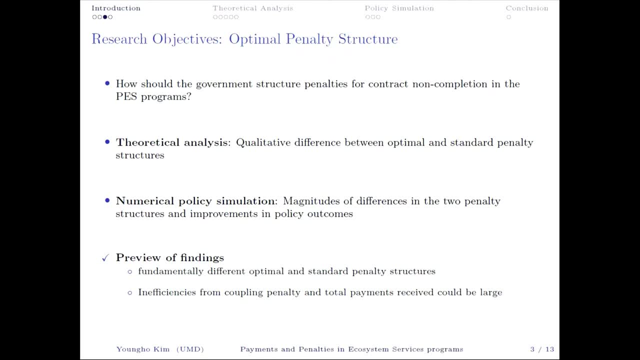 and compare it with the standard existing penalty structure And we're going to combine the theoretical result with the existing policy parameters to conduct numerical policy simulation. And the focus is we want to examine the magnitude of differences between the optimal penalty structure that we drive and then the standard existing penalty structure. 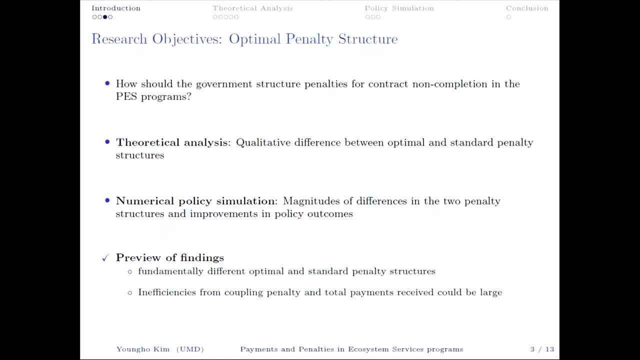 And then the next step is, you know, compare the net policy, net program benefits under each penalty structure and see if the difference is significant. And here's a preview of findings: We find that optimal penalty structure and standard existing penalty structure is fundamentally different. 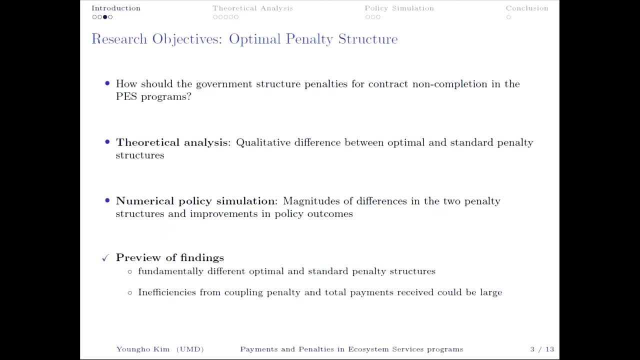 And we find inefficiencies from standard existing penalty is pretty large. So when you think about the standard penalty structure, it directly ties penalty to payments right. So you need to pay back what you have received when the farmer terminated the contract. So this coupling penalty. 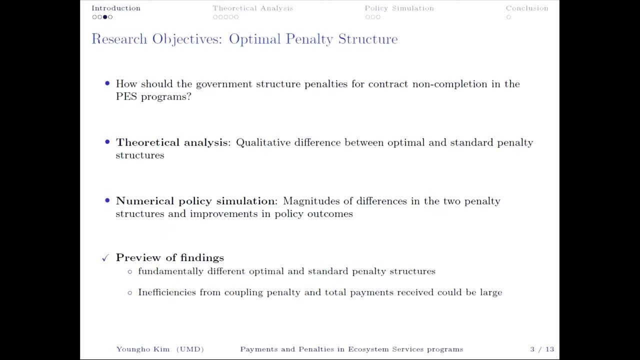 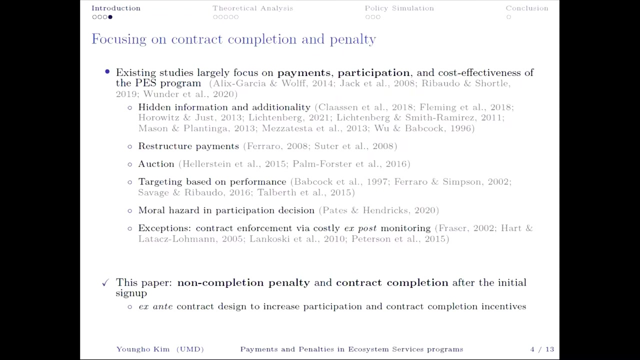 with total payments could be really inefficient if you think about any payment increase to encourage farmers' participation in these conservation policies can create simultaneously increase in penalty which again undermines the participation incentives. So I want to point out that inefficiencies from this paper. I want to briefly talk about existing literature. So existing studies have been largely focused on 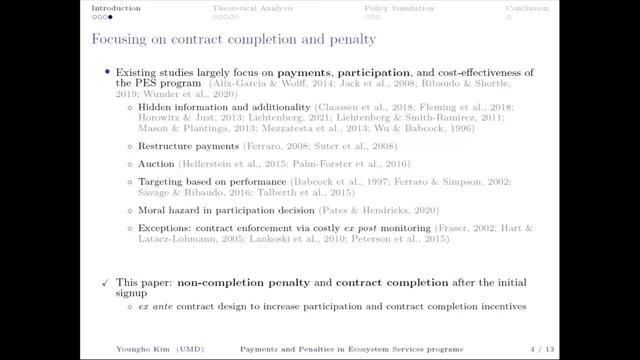 payments, how to restructure payments and how to allocate payments to different heterogeneous landowners or farmers to increase the participation of farmers in these conservation policies. So, for example, if you look at this slide, you can see that there's a lot of information about 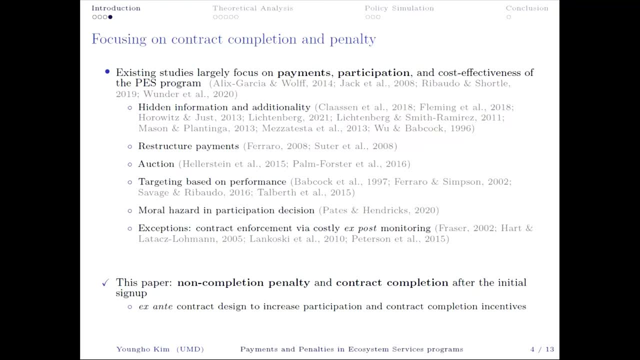 how to increase participation rate or cost effectiveness of these PES programs. right, But then our paper is focusing on penalty rather than payments, And also we're focusing on contract performance after the initial sign-up. okay, So the initial participation is not the end of the. 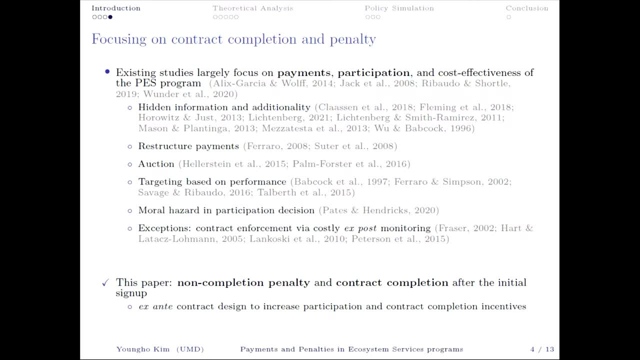 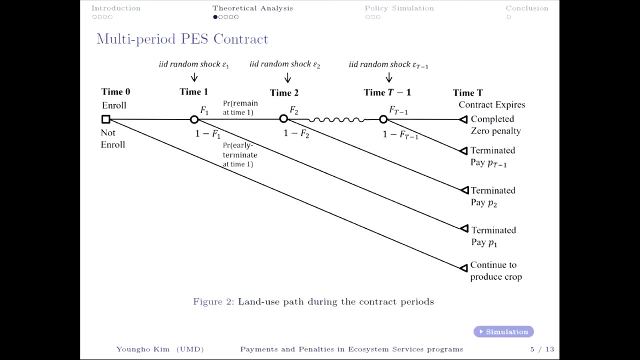 survey right, Because the contract is usually five to 20 years long and, even though many people sign up the contract, if the contract performance is low, then the cost effectiveness of these programs are pretty low. So I want to briefly talk about the multi-period PES contract that we consider in the model. 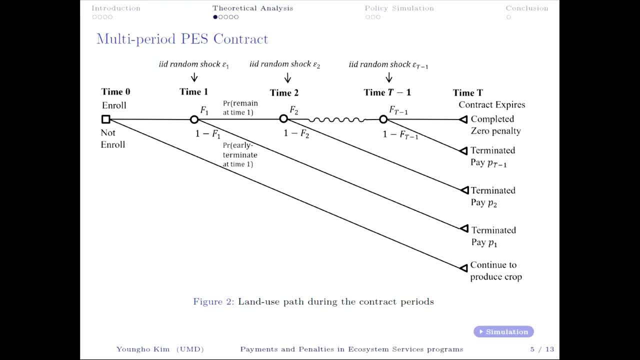 So at time zero. eligible farmer considers risk neutral. farmer considers the enrollment participation decision. So they have initial expectation on crop return during the contract period And if they do not enroll in the contract then they continue to produce crop. And if they enroll in the contract, only if the expected benefit expected return from program. 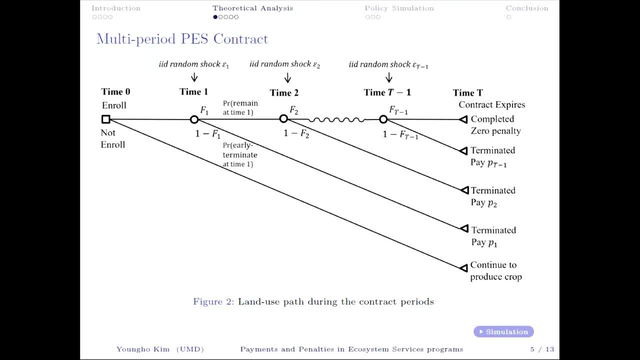 enrollment is greater than crop production, right, Then they are required to install the practice- conservation practice- and receive off-farm payment, and first annual payment And then, from time one to time, capital t minus one. there's a random shock that affects 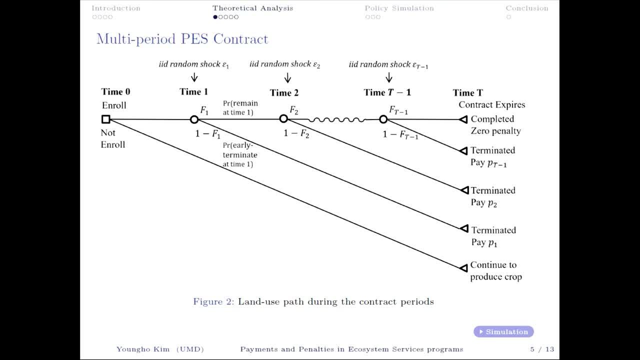 that alters farmer's initial expectation on crop return during the contract period. okay, nihilists yg in this. Does that impact the yield over in the first half or in the hightimes northern Minnesota- which is a huge reason for sustainability, but also will change the then consumer's initial expectation on crop return in the contract period? Okay, there's a spike in crop و. 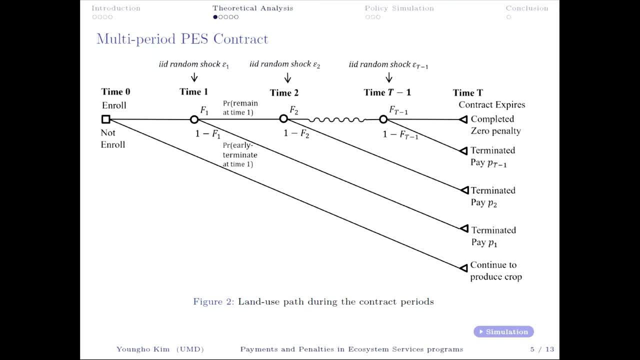 throughout the contract period, okay, and then, and then that the density of the random shock will create probability of contract termination and and probability that the contract is maintained throughout the country. and then that that's going to be repeated at each time and, in case of contractual determination, the panel, the farmer- is required to pay for the penalty. and then and 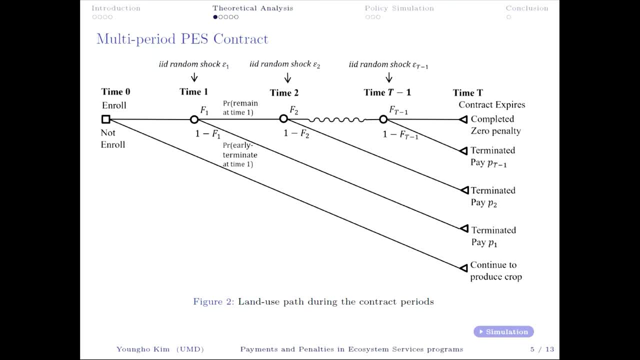 then that penalty schedule is from p1 to um p, capital t minus one over there. so so this, this, this random shock, is the only random shock. epsilon is the only random component in our model and and i'm gonna shrink this decision tree into one equation now to to talk about participation condition. so so this is the. so don't get. 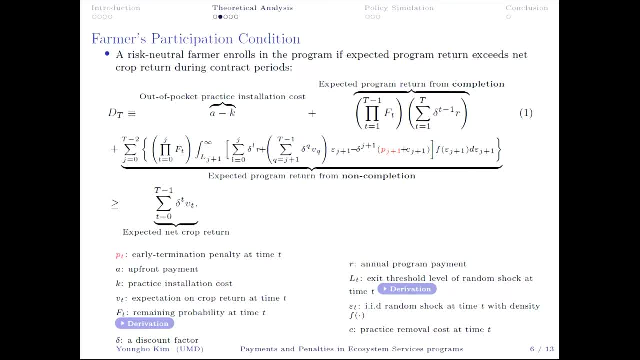 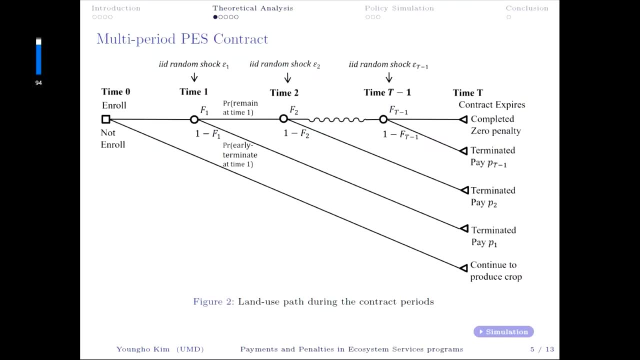 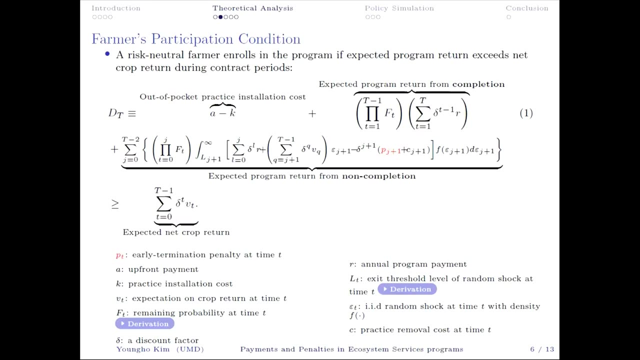 intimidated by this equation. so so left-hand side is just um expected program return, probability weighted. so there's a probability of contract termination and contract completion, right? so so this equation? what this equation shows is probability weighted summation of program return in case of contract completion and contract non-completion. okay, so that's just left-hand side. 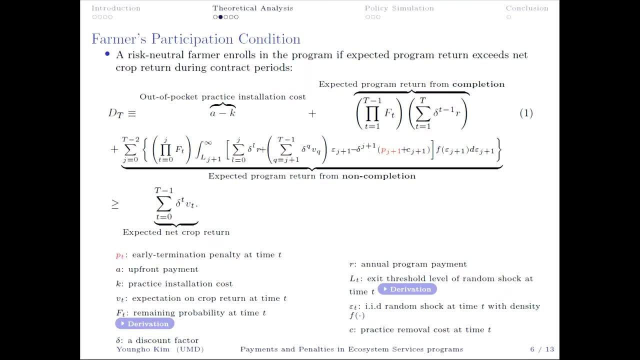 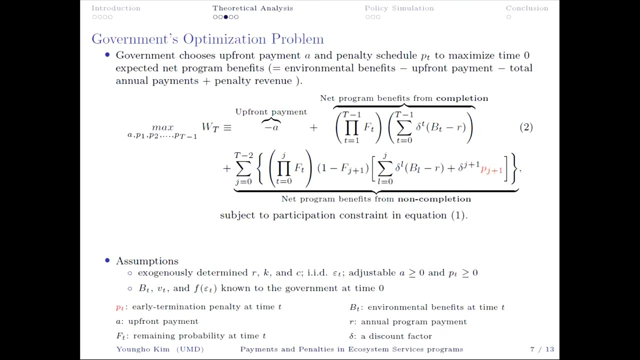 and the right-hand side is the total했습니다 expected crop return. So we're considering risk neutral farmer and they're comparing expected return from each option. And then there's a government optimization problem which is to maximize environmental benefit, less program cost plus penalty revenue. 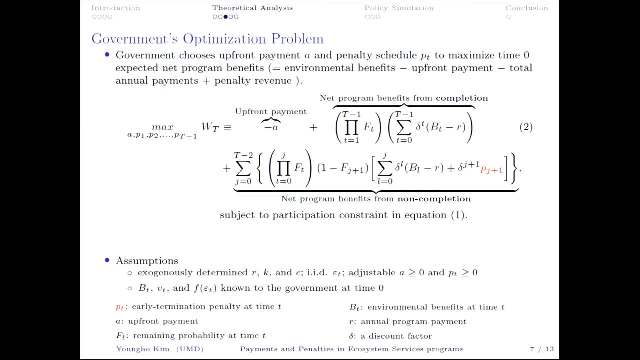 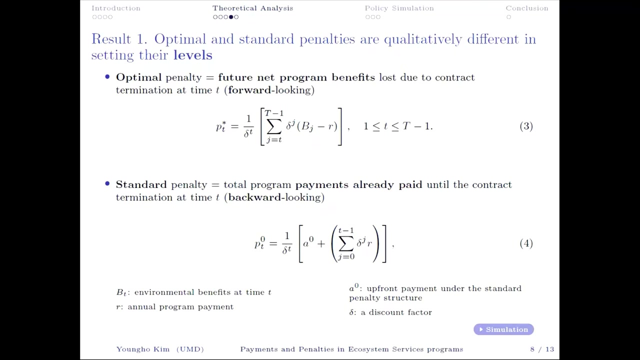 This is gonna be net program benefits that we're considering And they're choosing upfront payment and penalty schedule from P1 to P, capital T minus one. And this optimization problem, solving this optimization problem, will give us the first theoretical result And that is optimal. penalty structure is equal. 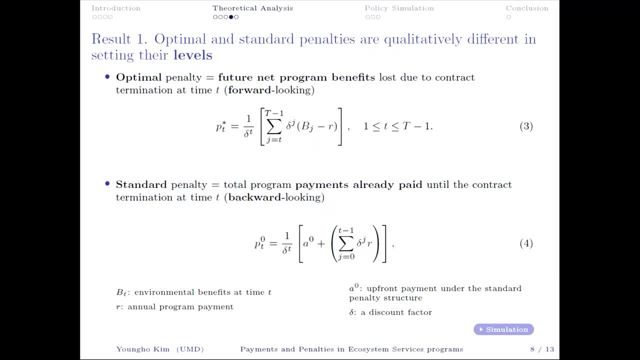 penalty level is equal to future net benefits lost due to contract termination. So optimal penalty structure considers future benefits, future environmental benefit lost due to contract termination. So in that sense is forward looking. But standard penalty structure is only a function of total payments received so far. 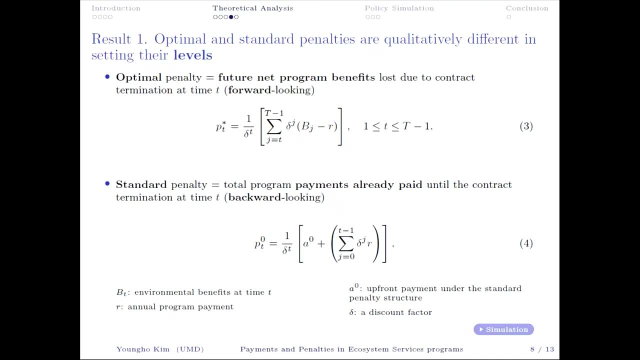 at the until the point of contract termination And in that sense is backward looking. So here I'm talking about how two penalty structures are qualitatively different in setting their levels. okay, And then now on a but. now I wanna talk about the trends. 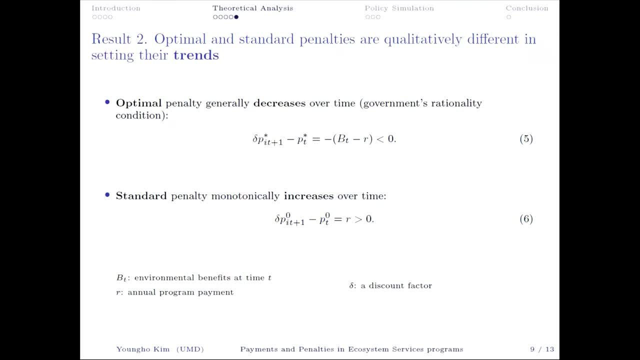 The optimal penalty schedule level generally decreases over time during the contract period, especially because the environmental benefit capital B is environmental benefit there And then environmental benefit less than the annual payment here. That is likely to be positive if the government implements the PES program. 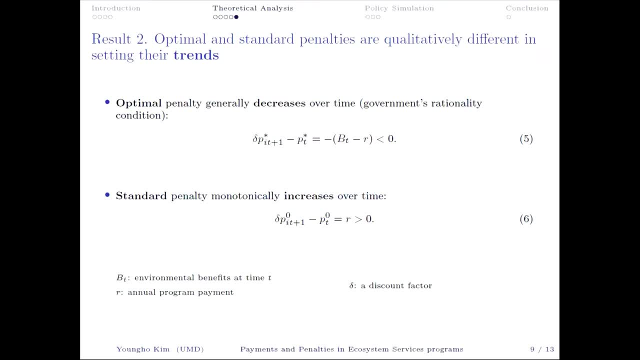 that generates net positive benefits right. On the other hand, the standard penalty structure monotonically increases over time because the annual payment they, the farmer, receive accumulates over time. So here I'm talking about the qualitative difference between the two penalty structure in setting their trends. 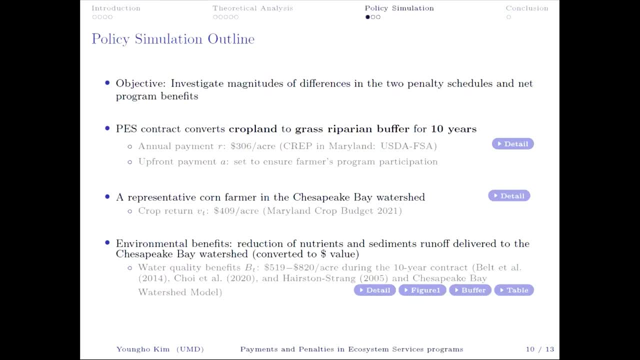 And then the question is whether or not this qualitative difference in penalty structures lead to quantitative differences, quantitative difference in the two penalty schedules and also net program benefits. So we're investigating magnitude of differences in the penalty schedules and also net environmental benefits And we're considering PES contract. 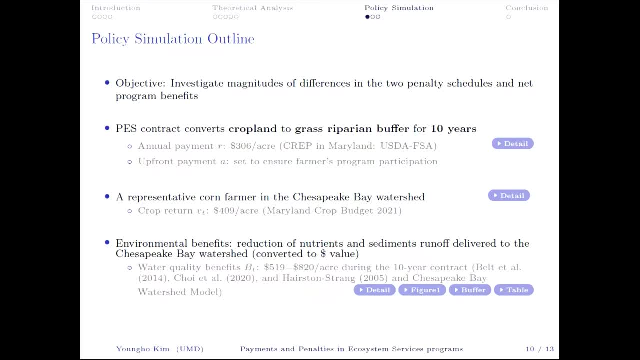 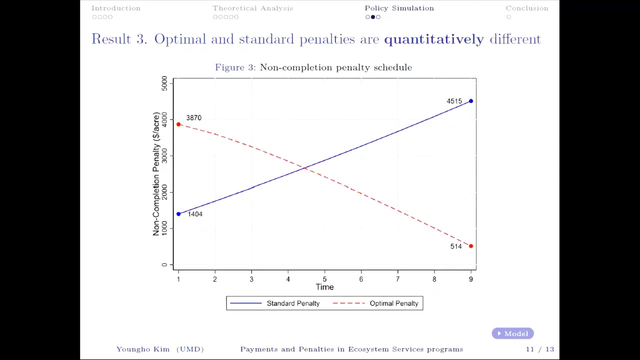 that converts crop land to grass buffer for 10 years, And we're considering representative home farmer in the Chesapeake Bay region And environmental benefit we're measuring is that reduction of nutrients and sediments runoff and delivered to the Chesapeake Bay. So this is the first numerical policy simulation result. 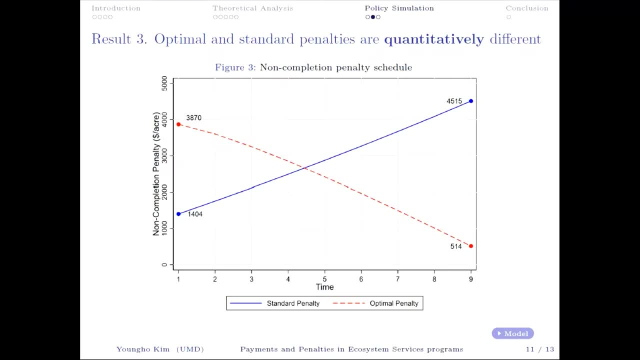 And the blue line is the standard penalty. So standard non-completion penalty monotonically increases over time more than triples here. So you can see here the reason is all the annual payments farmers receive increases over time. So yeah, it's just. 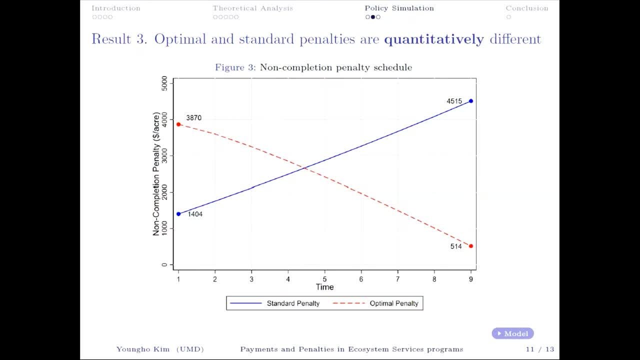 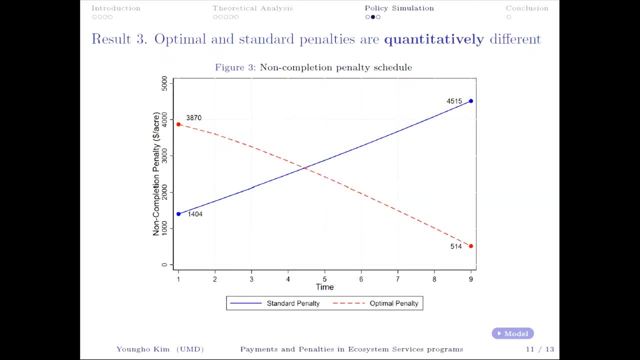 And that's decreasing over time. And that's decreasing over time. And if you think about qualitative aspects of optimal penalty when the farmers terminate the contract in the last period, right then what government loses is just one period of environmental benefit, less annual payment, right. 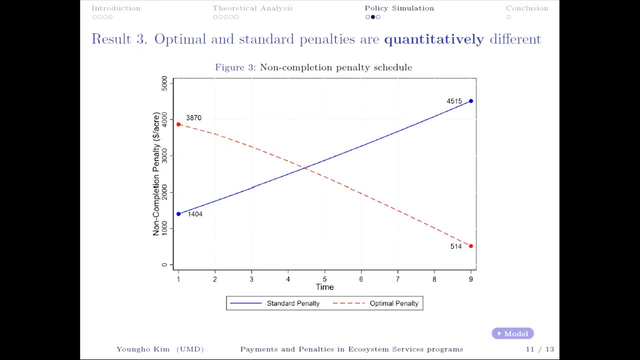 So net environmental benefit loss due to contract termination is small and at the end of the contract or closing to the contract expiration date- Expiritation date- Expirification date- Expiriation date. So we see the two penalty structures are fundamentally different in levels and trend here. 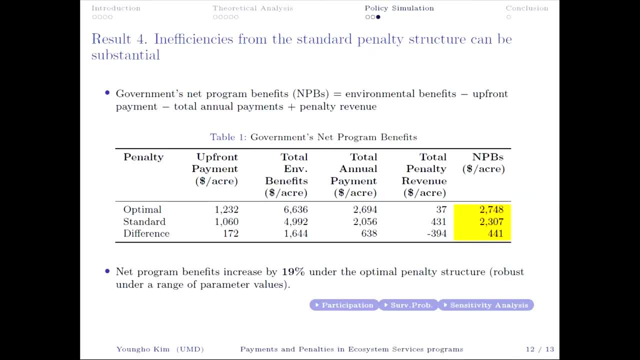 And then I want to talk about net program benefits. So the second column, off-rump payment, is the amount of payment that ensures farmers' participation in this program And that is greater under the optimal penalty structure, which means that farmers are more disincentivized under the optimal penalty structure. 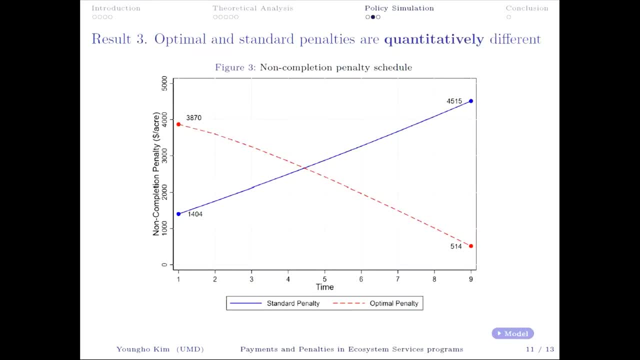 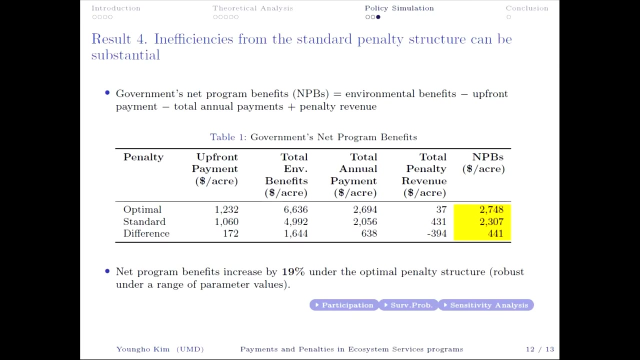 And the reason is obvious here. The penalty is high off-rump. Optimal penalty is large off-rump. So farmers are disincentivized to enroll in the program. So the government has to pay more to them to bring them into the program. 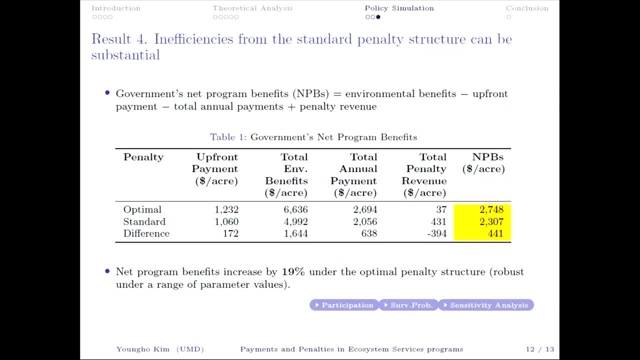 But the total environmental benefit is much greater under the optimal penalty structure because the standard penalty level is very low in the all-year contract period- right, And that's going to increase contract non-completion in the all-year contract period- okay, And as a result, the annual payment expenditure is lower under the standard penalty, but the penalty revenue is greater. 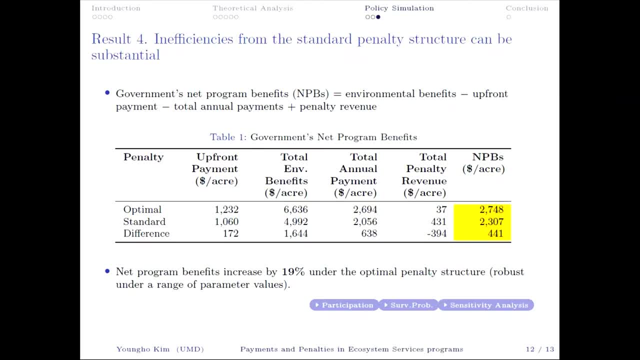 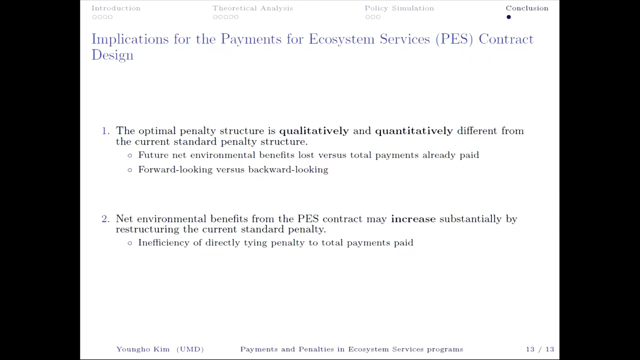 So I mean combining all the aspects, all the components: net program benefit increased by 19% under the optimal penalty structure. So this is the main result And let me wrap up with the two main takeaway message here. So from the theoretical result, 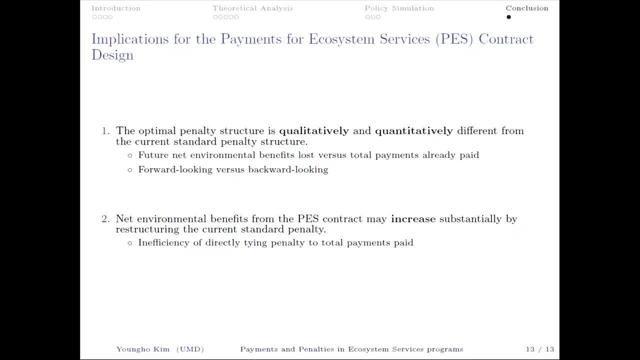 From the theoretical analysis we showed that optimal penalty structure is qualitatively different from standard penalty structure, right, And then that leads to quantitative differences in the two penalty schedule, as we saw. that cross-line in the previous figure. And the optimal penalty structure is forward-looking in the sense that it cares about future benefit loss due to contract termination. 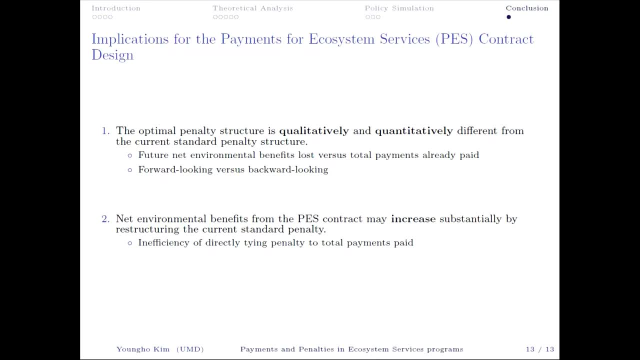 But standard penalty, Standard penalty structure is backward-looking in the sense that it only considers payments paid, already paid to farmer. And the second takeaway message is: direct coupling of penalty to payment is inefficient because any payment increase in conservation policy to encourage eligible farmers to 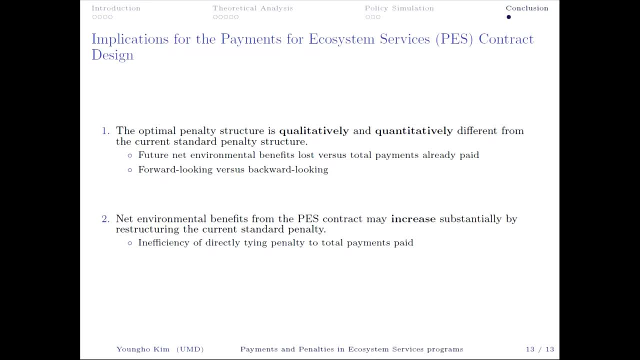 To participate in this program will simultaneously increase penalty level, because the penalty level is equal to total payments amount And that's going to undermine The participation in increasing participation in incentive due to payment increase right. So with the conclusion here is that N? assuredlysidevineinvolvement benefits from the pSo, ultimate development of benefits from the PS contract may increase significantly when we just how manyãosustant bankerate just currently increase. 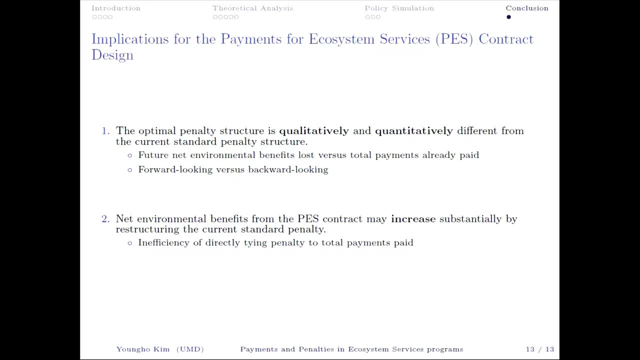 Here is what I should add for is what I should add for when we just restructuring the current um standard penalty structure in the in the crp, crab, equip and csp um those major farm bill programs. i think that's um all. i have thanks for the attention. 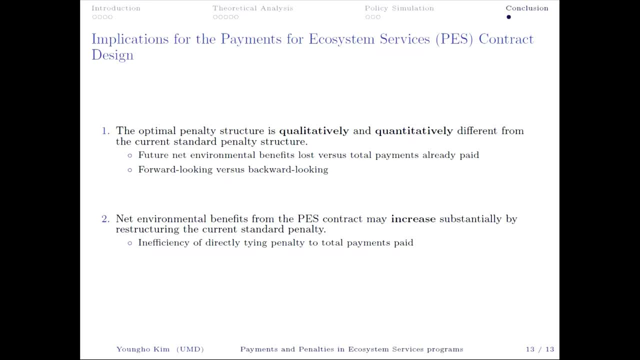 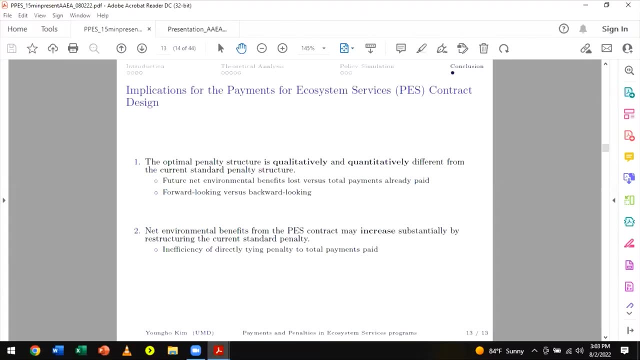 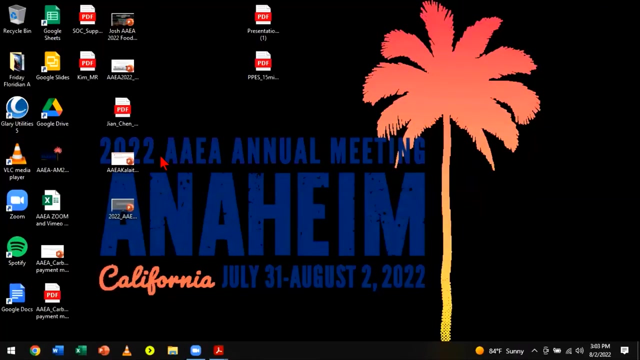 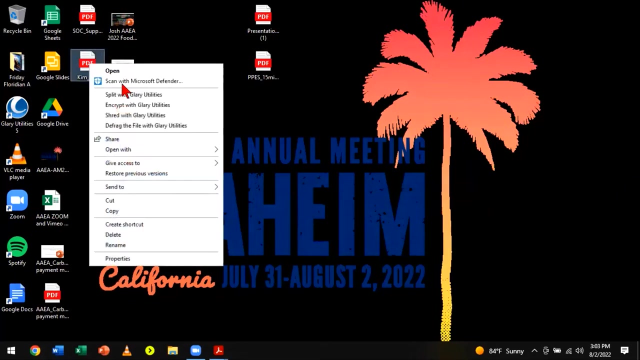 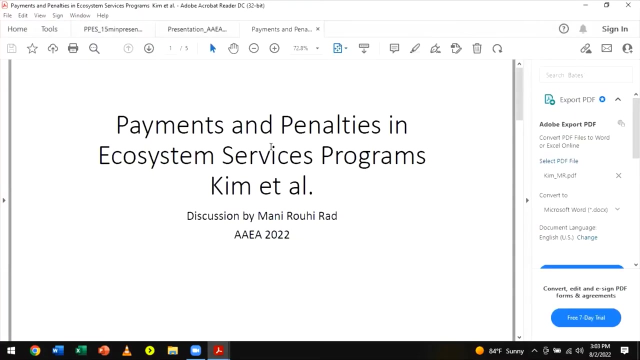 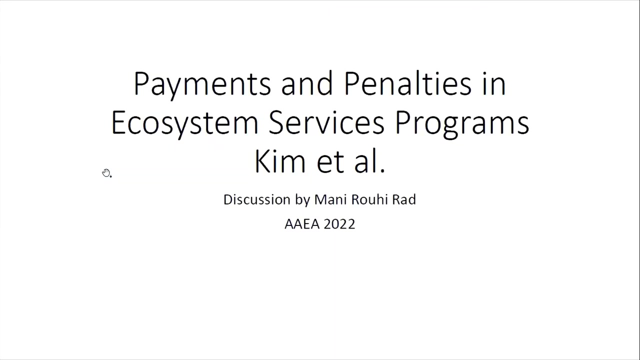 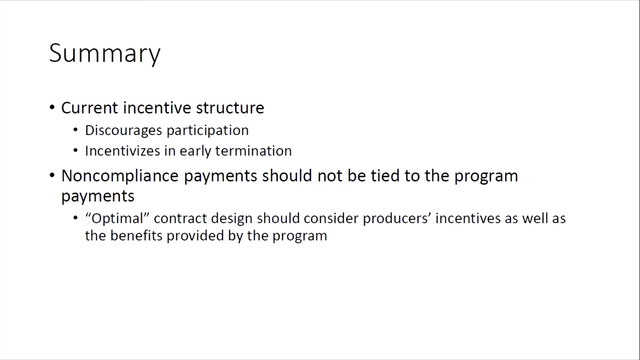 thank you, so foreign, okay. so yeah, i'm the discusser, mani rojira, assistant professor at texas a m university, and so i really like this paper. i think the? the message is very intuitive. i think the the message is very intuitive and very clear when you read the paper, and that the current incentive structure, the 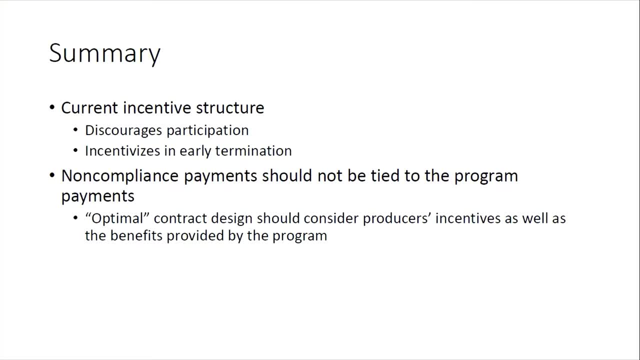 way it is set up discourages participants from participating in the program, and when they participate in the program, they want to get out of the program earlier, because the later, the more they stay, they are going to pay more. So they want to get out at the beginning and that is when the benefits are going to. 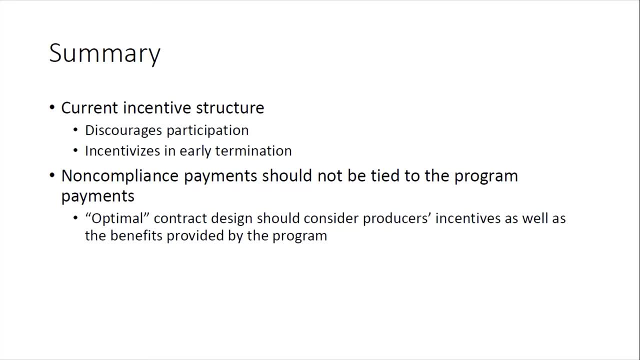 be realized actually going forward. The current structure, in a way, is very ineffective, because now you have to pay based on the history of the amount you receive, which is totally counterintuitive. and this message is laid out very effectively in the paper and I really like that: that it's very intuitive and it's 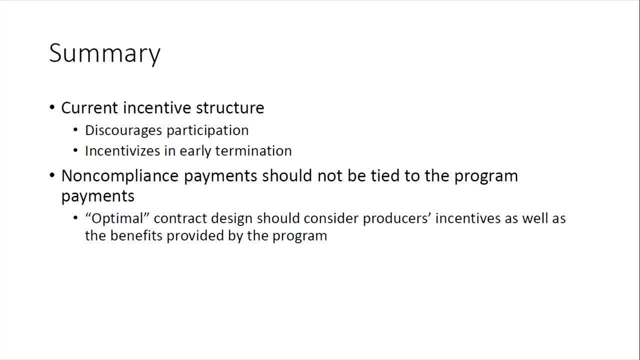 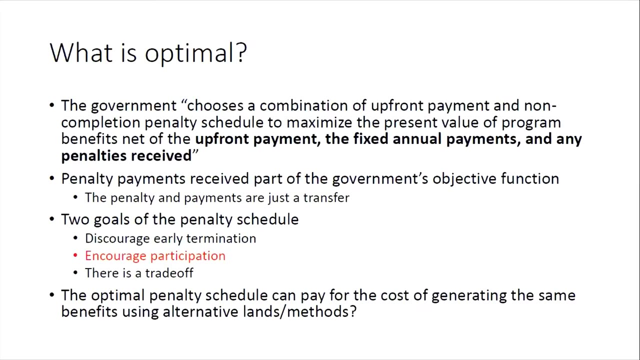 very easy to understand. Now, the optimal policy design, as I put it here, looks forward right, But then I think about it. I think about what is an optimal policy design, and this is what I was trying to think about as I was reading through the paper. 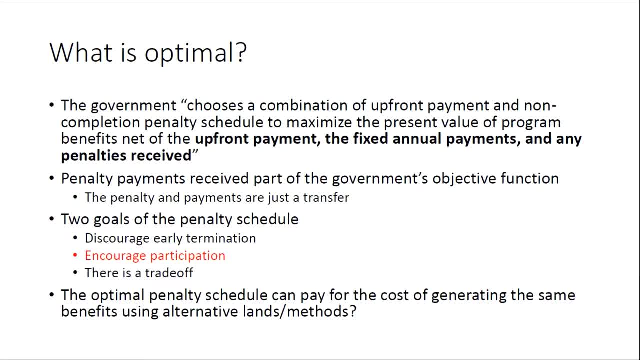 From the point of view of the government. so this is one of those last slides that the objective function for the government is that upfront payment minus the fixed costs and minus the penalties received. And when I think about the government, I think of the government trying to maximize social. 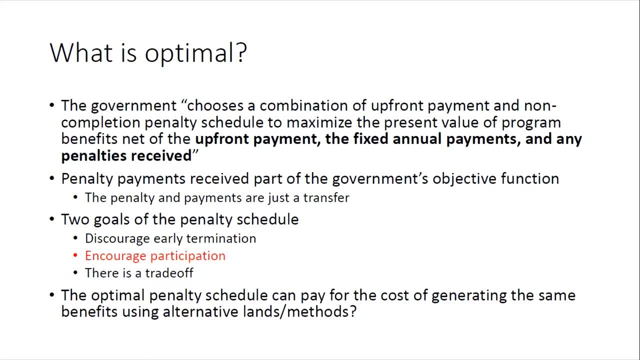 welfare in a way that the cost of the participation is the lost profits due to participating in the program and the benefits of participation and the benefits that are provided from environmental benefits generated. So for me the objective for the government really should be that the net benefits in 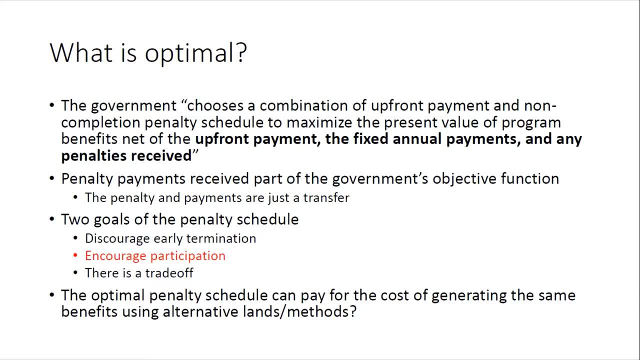 terms of benefits generated and the opportunity cost of that land participating in the program, So that this type of policy the optimal. so any of the money that is transferred from the participants to the government in terms of penalty, and any money transferred from the government to the participants is overall a transfer that just cancel out in the social 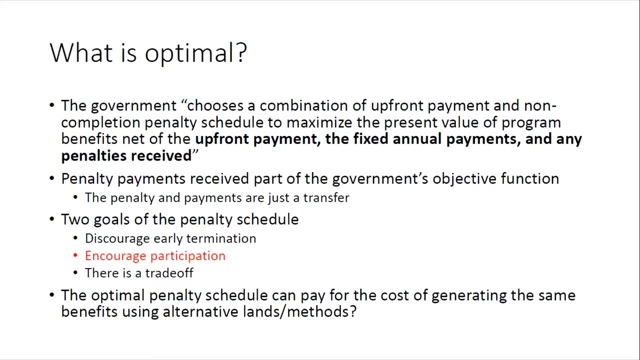 welfare function right. They all cancel out each other. So for me those are not an important part of the optimal policy design. And that becomes important because towards the end, when you discuss what is efficient and what is not efficient, efficiency for me is that social objective function, that 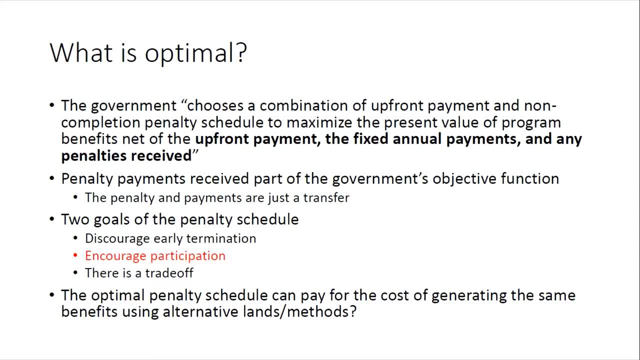 maximizes the social welfare. But then that becomes very interesting there that the objective, the objective, function in a way we can. if you have everyone already participated in the program, if we set the penalty very high, nobody will get out of the program anymore. 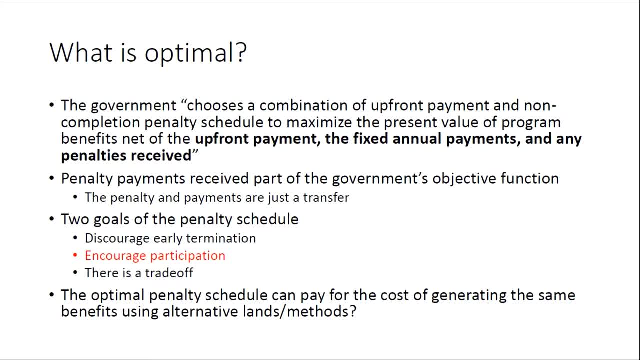 So they are locked in. They have to pay millions of dollars if they decide to get out of the program. So they're already locked in, but what that does then discourages them from participating in the program. So there's a trade-off between encouraging participation and discouraging living of the 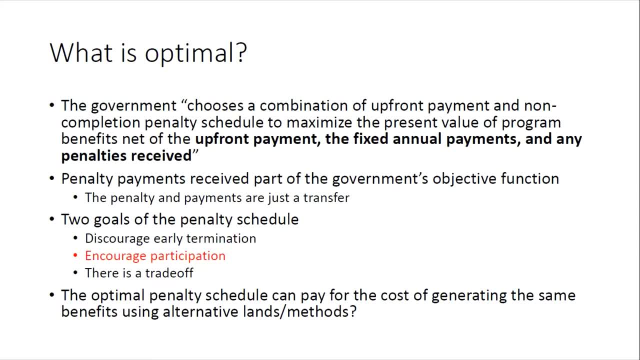 program And I think some of that- trade-offs- can be laid out a little bit more clearly in the paper in a way that I think about what is the extent of that market? How substitutable are different producers with each other? So if a producer leaves a program, they should pay the amount that the government will then. 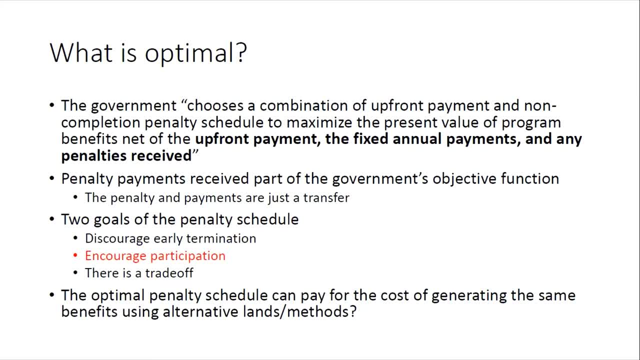 use to bring in the next best land into the program. So in a way, that is how I think about the government's problems: that the amount that you should be paying is the benefits you generated, but how much you need to the government needs. 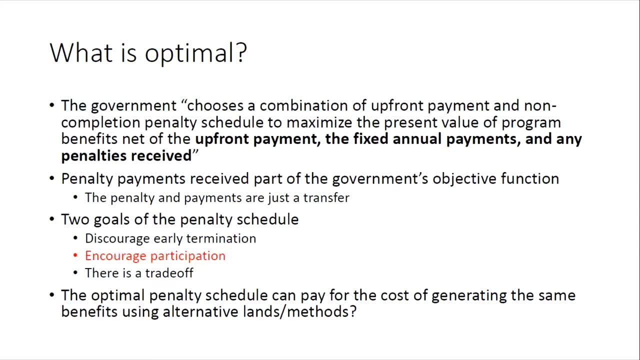 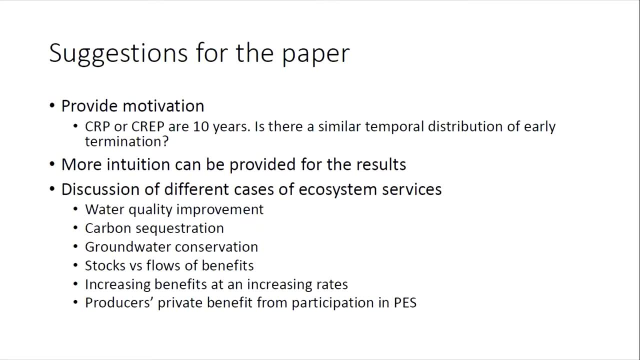 to receive, to generate the benefits from an alternative secondary, They can alternative source that generates the same amount of benefit. So that is kind of the bigger picture type of thing I could point. I had about the paper that kind of my thoughts. I had some more minor thoughts, if you will, about the paper. 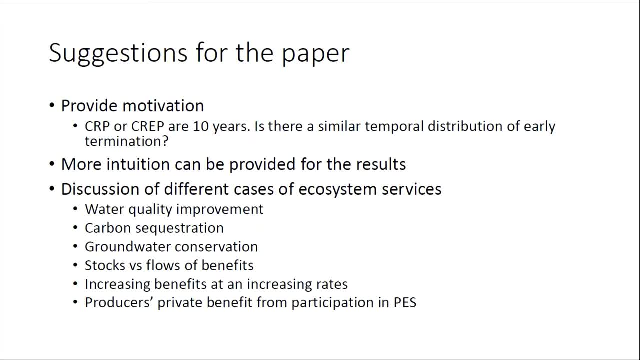 how to as I was reading through the paper. okay, just quickly that I say that, in terms of the motivation, there are programs like CRP or CREP that are 10 years and would be nice to see whether we see individuals leaving the program in the first couple of years. 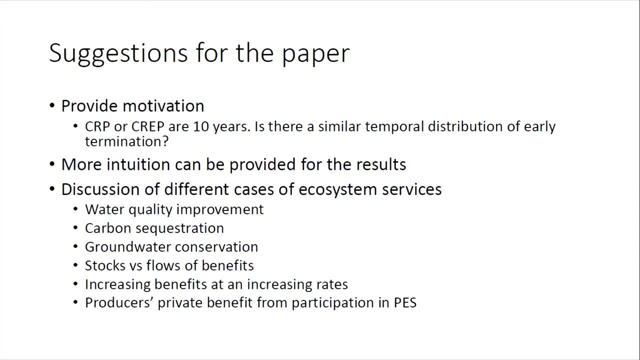 or they actually did. So I think that's one of the things that we need to be thinking about in terms of the distribution of the time that they leave the program And when you present some of the results. for some of the theoretical results, I think some 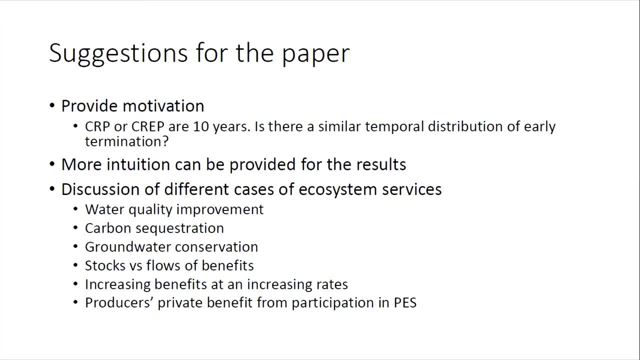 of that intuition might help as well. One thing that I think would be very helpful in laying out the paper would be that after you generate the theoretical results, it would be nice to say, okay, let's apply this to a few different types of ecosystem services that are very different. 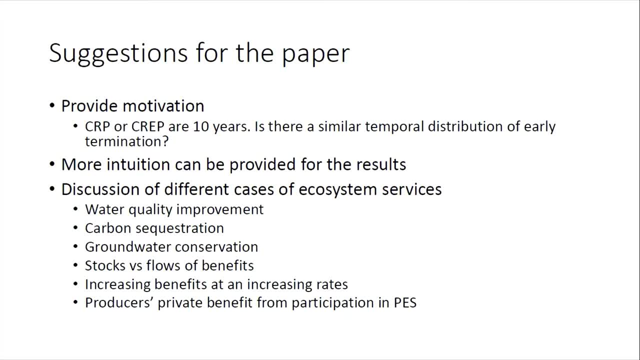 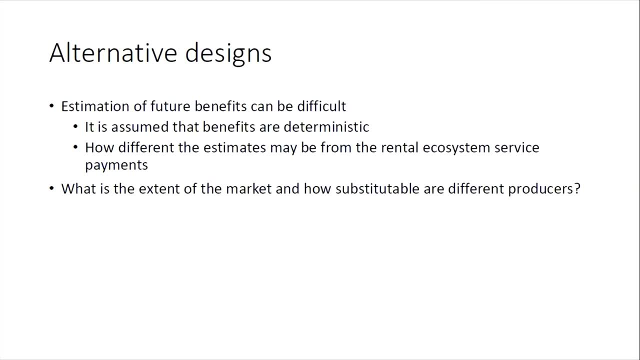 Some of them are stocks, some of them are flows, some of them generate benefits over time because they are stocks, But some of these show that the payments, the penalty structure, is very different across these things. So that's basically, and the last point that maybe we can discuss later is that this rental 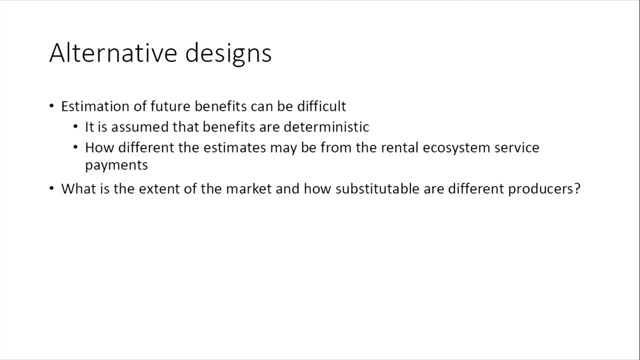 model of ecosystem services, that what if I pay you for every year of the benefits you generate? that this kind of like carbon sequestration type of literature that they're thinking about is what if we rent carbon ecosystem services from the producers? It is stock, but we are renting them from the producers. 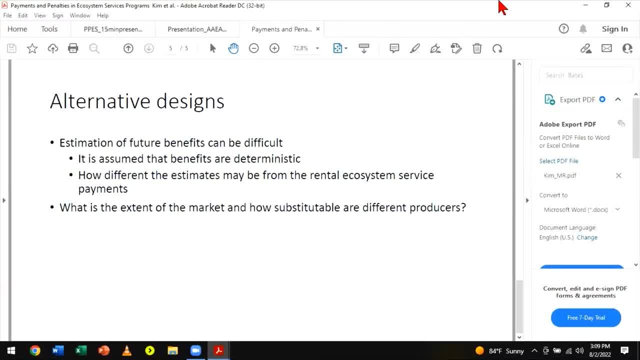 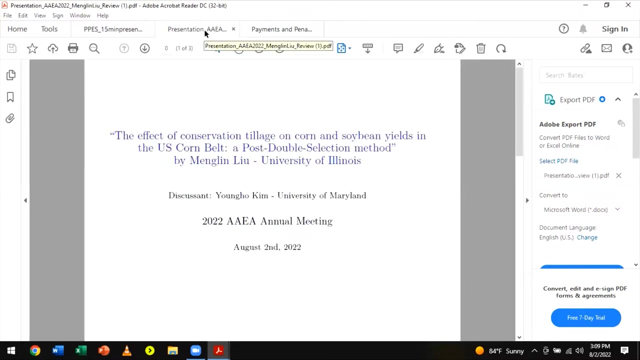 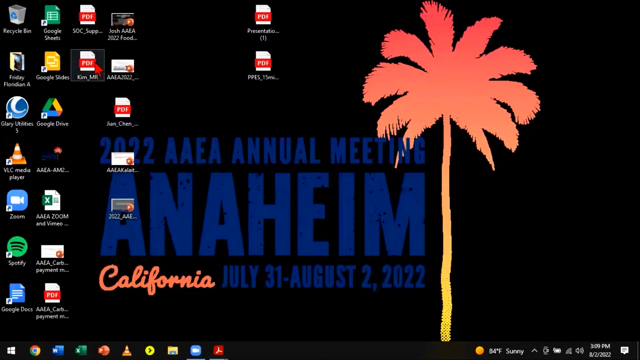 So those are my comments for it, Thank you. Am I the next presenter myself? Oh yeah, 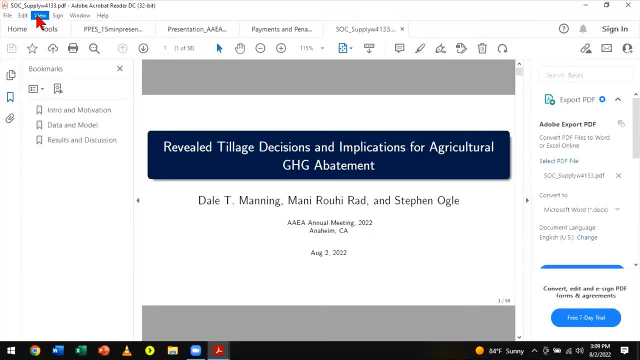 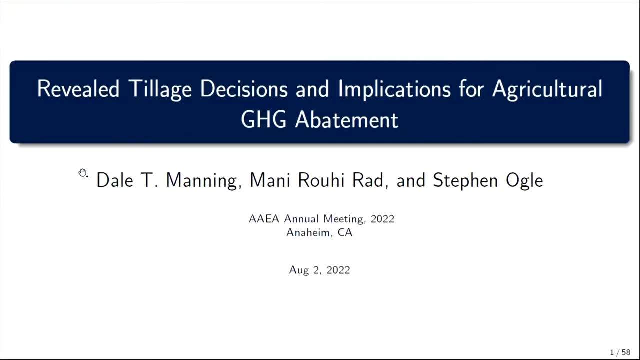 All right, I'm the next presenter, So I'm the second author, Marnie. The co-authors on this paper is Dale Manning, who is at Colorado State University in the Ag and Resource Economics Department, and Stephen Aldo, who is, I think, in the Soil Science Department, but in Colorado. both of them are at Colorado State Universities. 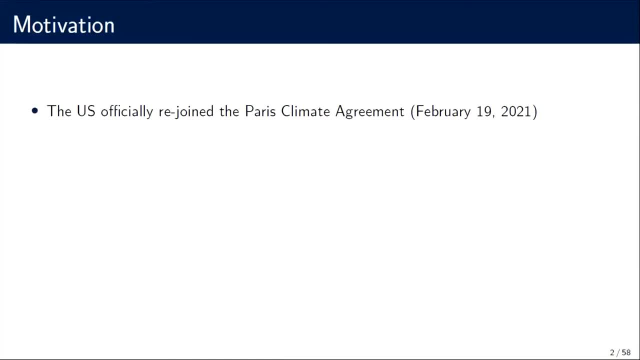 So, as you know, US officially rejoined the Paris Climate Agreement last year. basically, And part of this voluntary part of joining the Paris Climate Accord was that providing soil sequestration and climate services partly through agricultural and climate-smart agricultural practices. 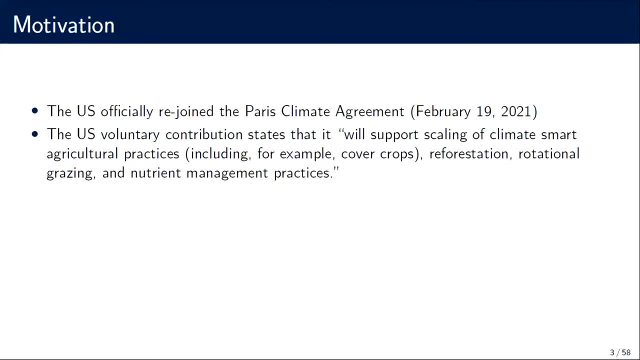 For example, through cover crops or tillage practices, or even restoration of certain agricultural practices and certain agricultural management policies. Okay, This type of agricultural practices can take carbon off the soil, the atmosphere and sequester it in the soil, But not only that, they can also reduce the N2O emissions, or nitrous oxide emissions, from the agricultural production. 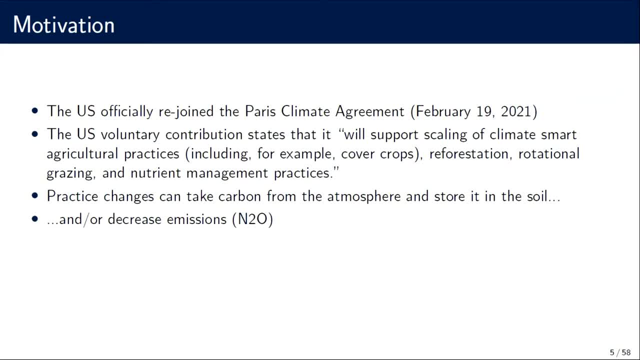 So they kind of provide two types of services at the same time, changing or modifying agricultural conservation practices When we look at some of the more biophysical literature on the potential for agricultural lands or for lands in general for contributing to this climate externality. 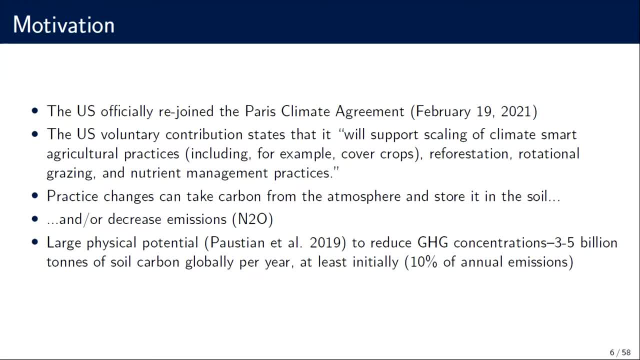 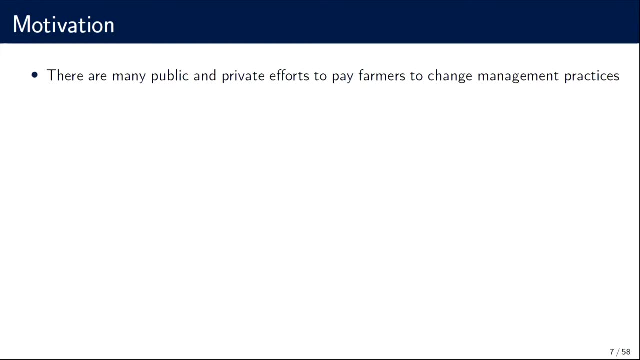 they suggest that there is a very large potential, in terms of 10% of annual emissions, for example, to be able to be evaded through agricultural conservation practices. But as we know- and as we know there are too many- there are many public and private efforts that are going on right now for contributing. 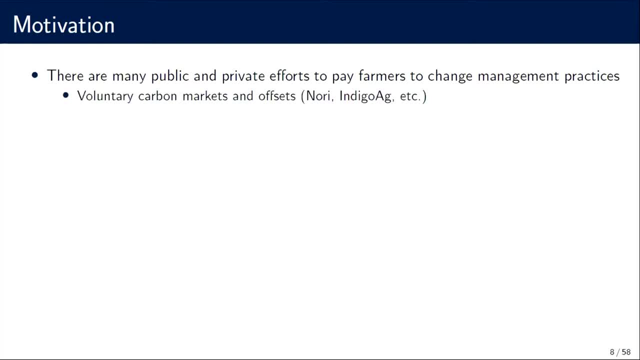 to this debate- For example, companies like Nori or Indigo Act- that they are providing payments, voluntary payments, to agricultural producers through carbon offset markets for them to implement certain practices to sequester carbon and to reduce their emissions. At the same time, we have lots of government support, technical support programs that are being implemented right now for agricultural producers that are incentivized through the government payments. 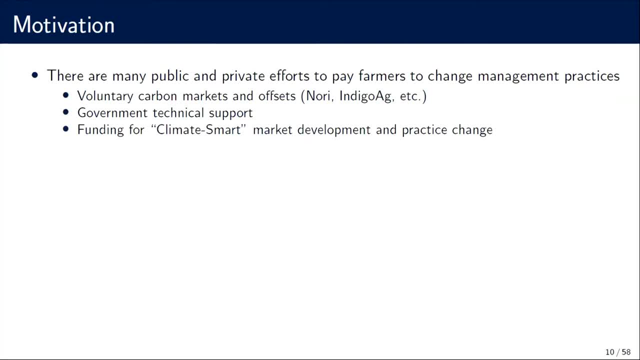 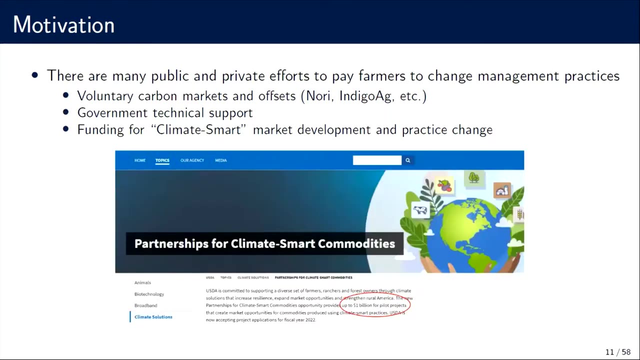 Okay, Thank you. So again, I think that additional inputnext in our actual Lex for a much easier existence to kind of provide a way to do that. Thank you very much. Great, Anyway. thank you so much, indeed. Thank you so much. 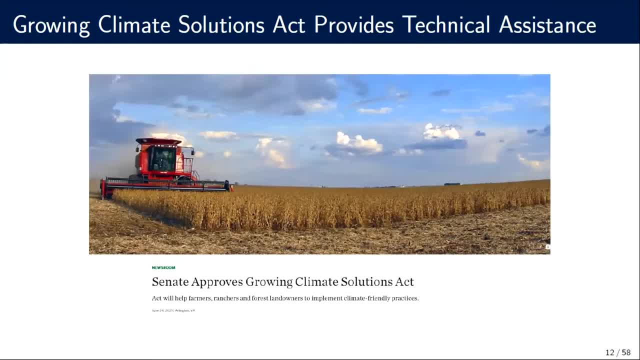 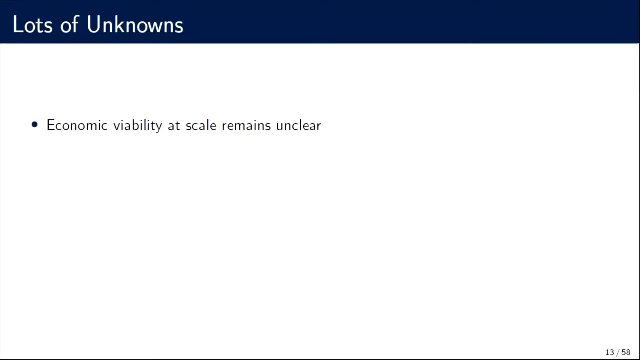 Thank you. That was a special climate solutions act provides technical assistance to agricultural producers for policy, for practices that will sequester carbon and reduce emissions from agricultural production. well, while there is, there seems to be a lot of scope, at least from the biophysical side. 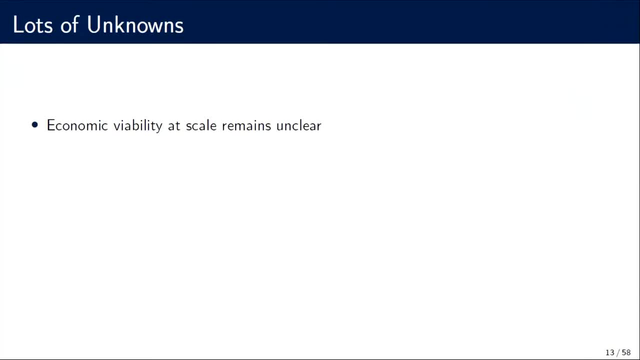 on the economy, on the potential for agricultural lands to contribute to this debate. when we think about the larger scale, whether these, actually these things can take place, when we think about the economics of it, the economic viability of it, still remains unclear. whether the potential physical potential exists and whether the economic potential exists are two. 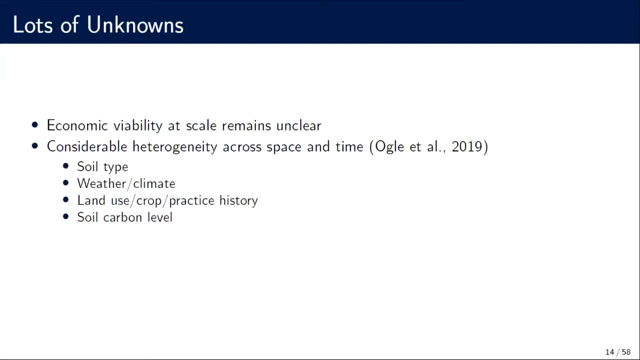 different things, and this is probably partly very important because of the significant heterogeneity that exists in a lot of agricultural lands, for example, in terms of soil type, weather and climate condition, the existing land use and practices and the existing land use and practices, history and soil carbon levels that exist already in the agricultural lands. 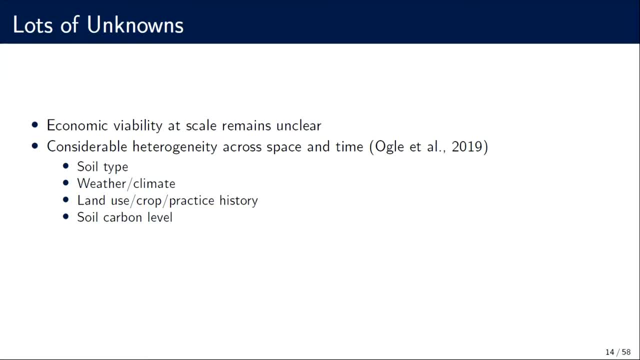 so it's really important to consider all these things and when we consider all this heterogeneity, we may not have- we may not have as much potential as we think in agricultural lands and besides that, literature have shown that these changes in soil, carbon sequestration services may. 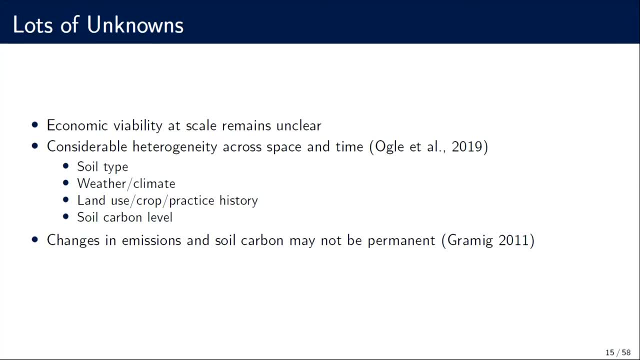 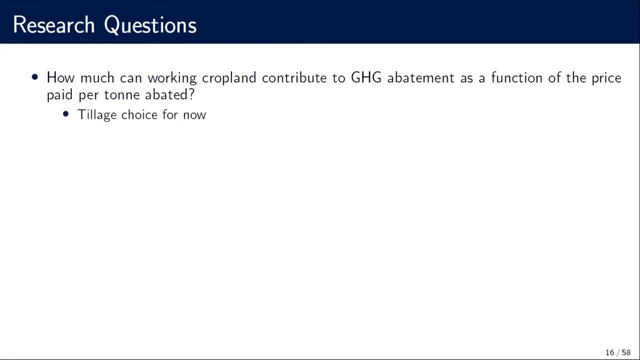 not be permanent. for example, agricultural producers who participate may leave these programs, or maybe there is leakage in terms of the amount of carbon sequester. so we have two objectives really in this, in this research. we want to first an empirical question that we want to look at is: 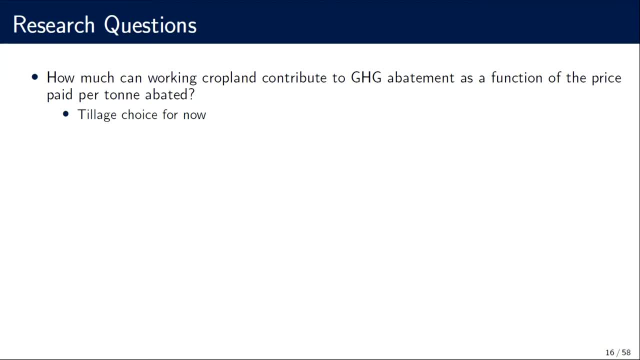 how much can working agricultural lands contribute to the ghma abatement policy question as a function of the price of carbon that will be paid to agricultural producers? and there are different ways to think about it, incentivizing adoption of different practices, but what we are thinking of here, at least in the presentation today, we are thinking: 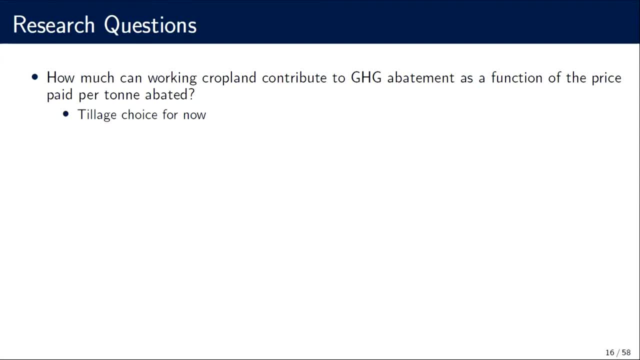 about tillage choices, for example, no till or reduced till as an alternative to full till. but also we have another alternative. here is we want to understand how do discrete choice models affect this empirical supply curves for a gh abatement services. so we look at different specifications, for example with or without different controls. but we are also interested 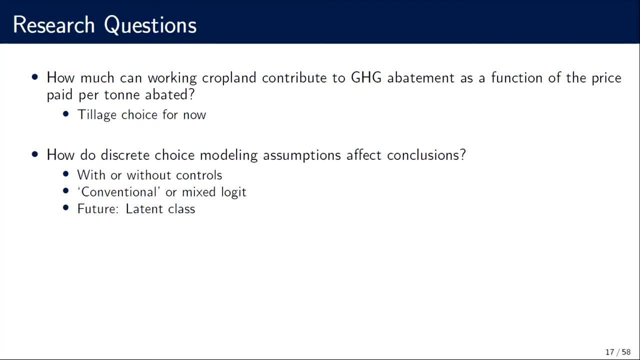 in this conventional or conditional logit compared to the mixed logic type of comparison and what that means for the flexibility or for the elasticity of that supply curve. in future we are hoping to do different types of discrete choice models and to be able to compare them together and see what their policy. 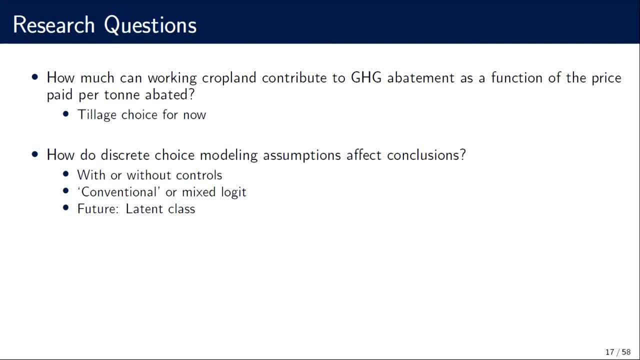 implications are for the supply of carbon sequestration services and into into our emissions. so what we are going to do is we are going to estimate the discrete choice model with the existing practices is that we have historically for iowa- and then simulate different policy simulations. 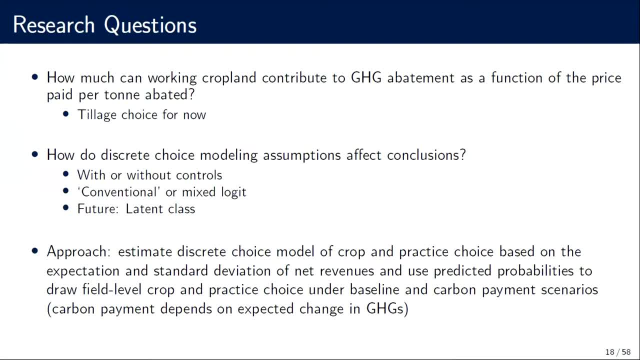 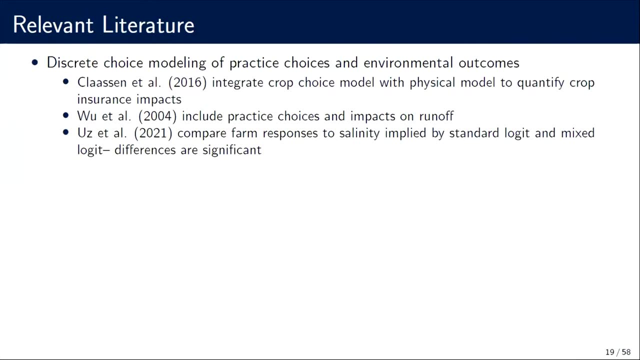 for different prices of carbon to be able to generate the supply curve, basically for provision of soil sequestration and into our emissions, for in general for carbon services. and there are two groups of literature. there is a more recent group of literature that studies the discrete choice modeling of carbon. sabe, Well, that's basically anything, because the 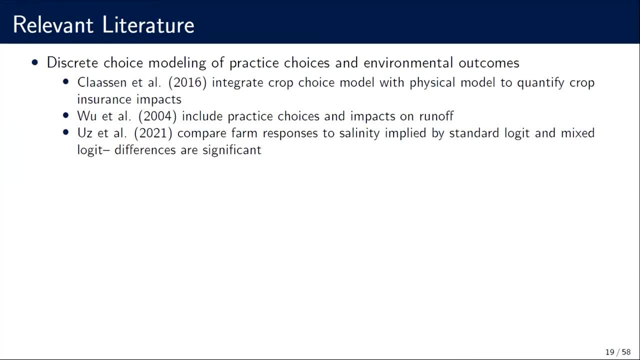 changes that are coming on the snow coast are- these are all things that are changing throughout the of crop and practice choices at the farm level that these studies use discrete choice models that kind of we are using the same multinomial logit or mixed multinomial logit type of models. 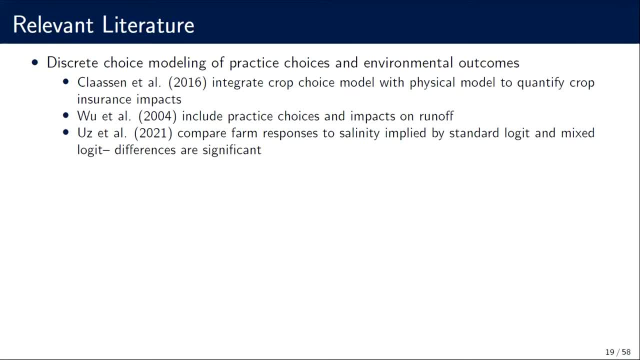 and compare the the outcomes of these models and the welfare implications of those. for example, one of the more recent papers by oz et al. they look, they compare the effect of salinity on crop choice decisions and they show that this heterogeneity is very important for understanding preferences. 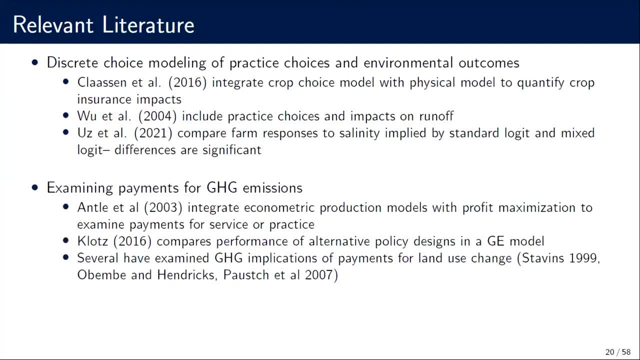 over salinity on crop choice. another group of literature studies the ghg. this is more of a ghg emission literature that model crop and practice choices. some of them and the other ones study the study, the preferences you model, the general equilibrium type of models and compare. 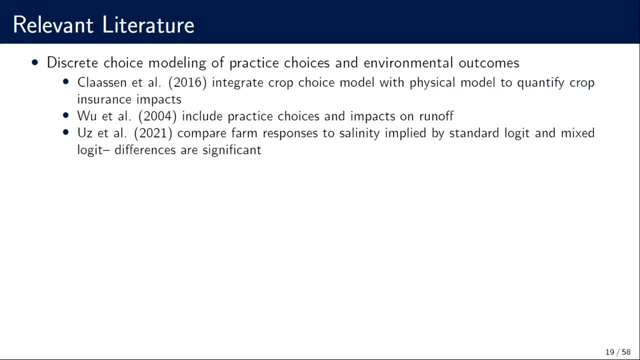 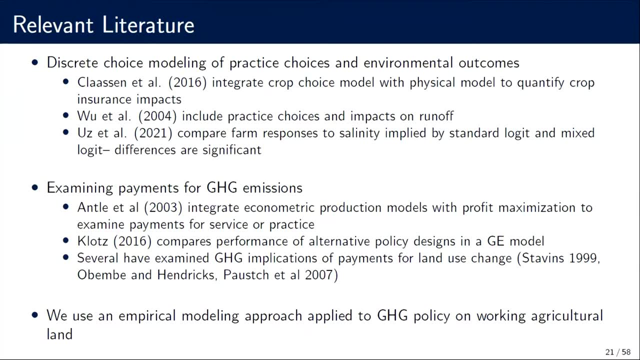 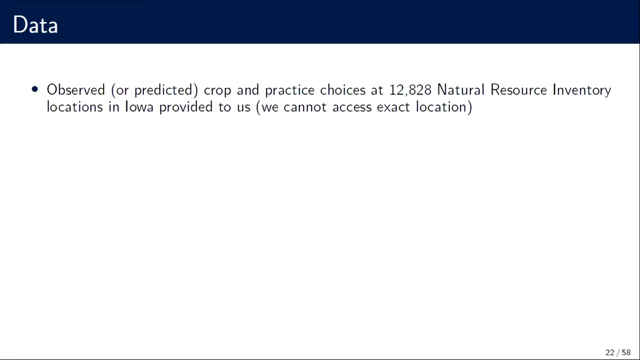 different types of policies. so we are going to use an empirical discrete choice model to model producers historical preferences through their historical decisions and then use simulations to be able to simulate the supply curve. The data that we are going to use are more than around 13,000 observations. 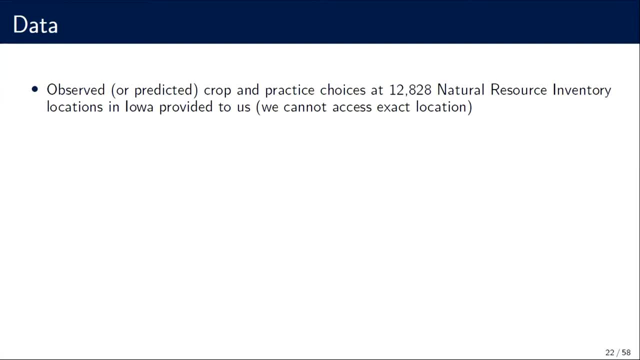 using the natural resource inventory, or NRI point in Iowa. This data is a panel data set, So we observe their land use choices. We also observe some form of their tillage choices as well. We don't exactly know what's their location. 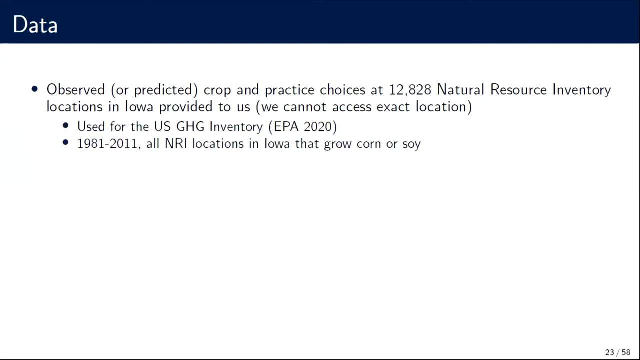 We know at this point we only know that they are in Iowa, but in the future we are going to know which county they are located in as well. So we know some spatial distribution of these points as well. But at this point, 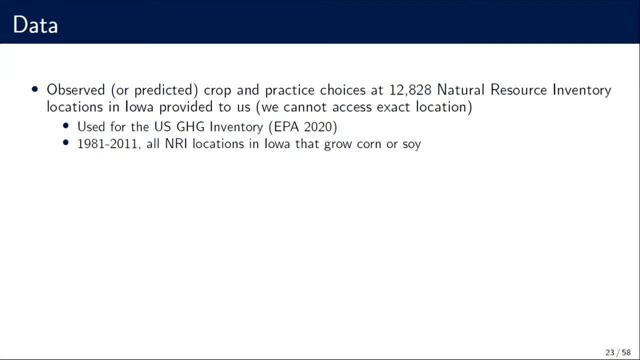 we only know that they are in Iowa and all our data right now is from Iowa. We are hoping to expand that to entire Corn Belt in the near future And this data and this modeling that we are using in this analysis is very, very important. 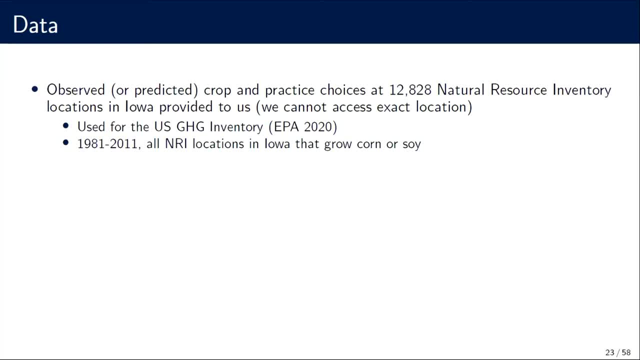 Because this data is used for reporting the actual emissions of the US to the IPCC and to the EPA. So this data that we have is used by the US government as well, And the data goes back to 1981. So we have around 30 years of the data. 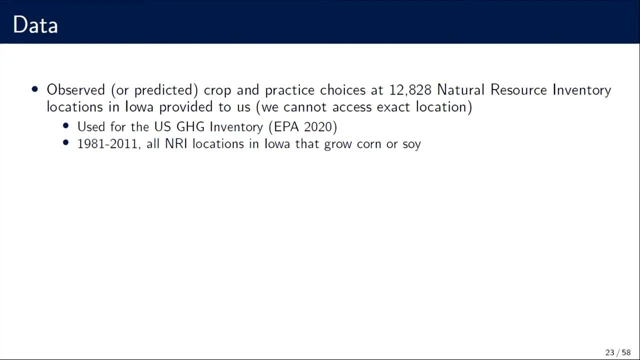 that for the producers that grow corn and soy, So we have more producers in there, but we only focus on corn and soy and tillage practices for now, And the variables that we get from this data set include crop choice, practice choice. 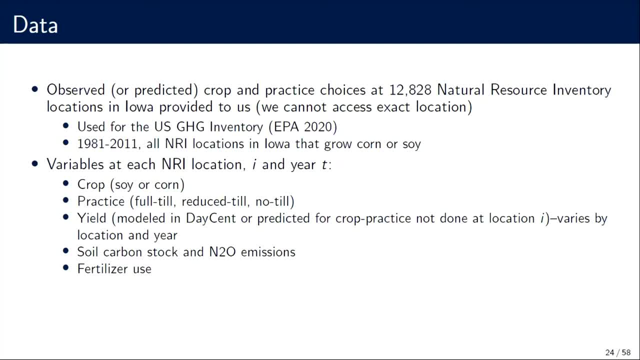 Their yields. that are modeled with the DASENT model, which is a ecosystem simulation type of model but is used for this analysis And we don't actually observe the yield- actual yields- at the parcel level- but this model, the DASENT model- that simulates 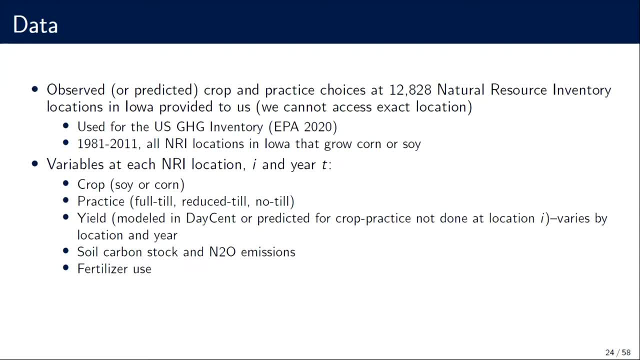 changes in carbon sequestration, changes in N2O emissions and the changes in crop yields. basically is used for analysis and also fertilizer use And we get the crop prices and fertilizer prices from the USDA data sets to be able to generate profitability of different crops. 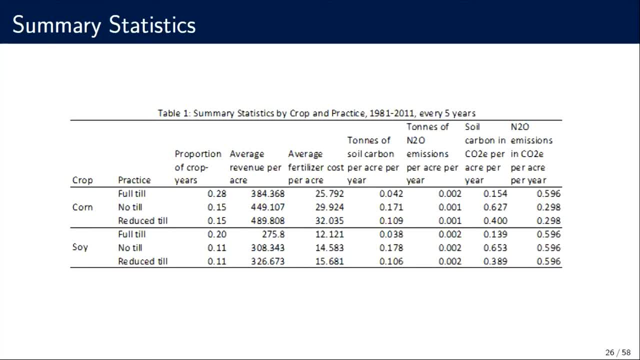 So, as I said, we have two main crops that we are going to focus on, at least for today's presentation for corn. that are corn and soybean, and three different practices: full-till, no-till and reduced-till. 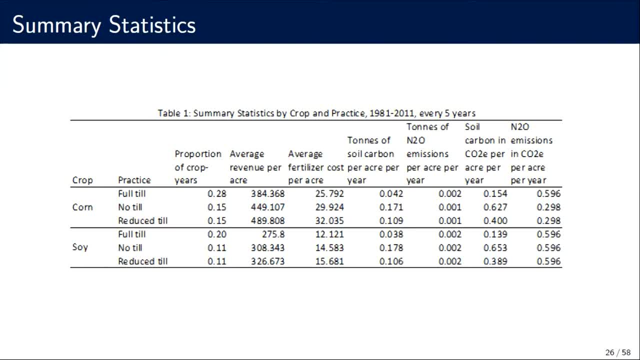 As you can see, most of the crops are full-till. for both corn and soybean There is variation in terms of this simulated revenue and fertilizer costs. So these are to understand these columns. these are simulated crop yields that then multiplied by the price of the crops. 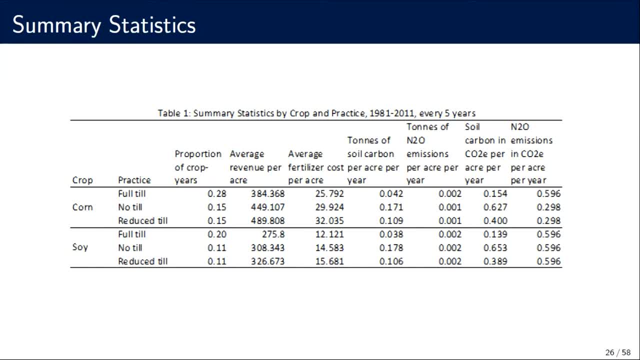 And these are simulated fertilizer amounts that are multiplied by the cost of fertilizer elements basically. So what we can see here is that full-till reduces both crop yield and also has higher fertilizer costs. In terms of fertilizer cost, it makes sense that tillage practices reduce the cost of fertilizer. they reduce the amount of fertilizer needed, but also that they keep moisture better as well. What we also see is that tillage practices tend to full-till practices tend to have higher emissions and lower carbon sequestration. 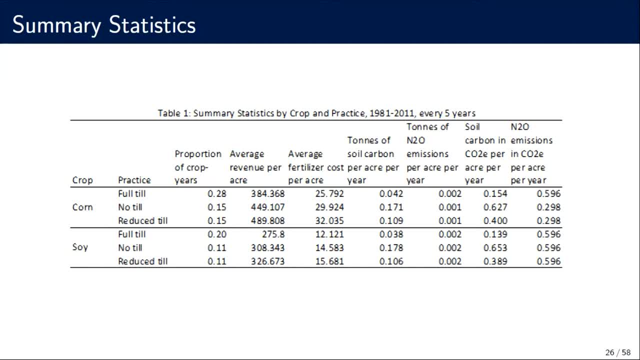 So if we incentivize, if we have more, we can keep the fertilizer better, But if we have more we can keep. you pay producers for if you have a price for carbon, we should see an increase in till, no till and reduced till and a shift towards noting and reduced. but what we also see historically is that 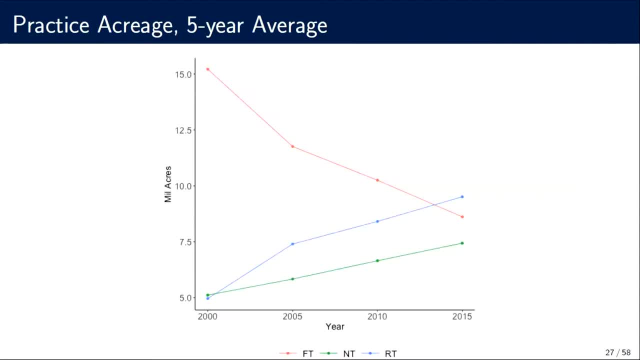 there has been an increase in no till and reduced tilling in the corn belt and, for example, in the state of iowa. so we see a reduced reduction in full till acreage and an increase in no till and reduced till acreage over time, and what that means is that we have we have had an increase in the. 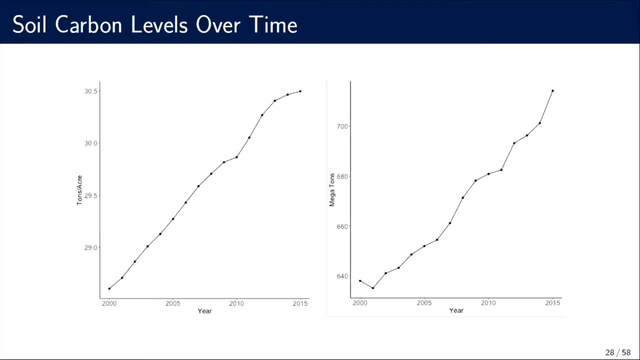 soil carbon sequestration over the past uh couple of decades and if you see this figure for the first time, that may look that is interesting- that it's not that we are depleting soil carbon resources, but because of both these conservation practices and also because of fertilizer use, soil 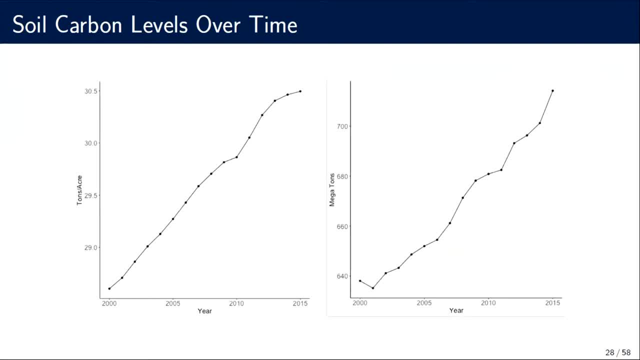 carbon. soil carbon has been increasing overall over time, but what that also means for policy is that if we incentivize the use of conservation practices, even in the baseline, we are seeing an increase. so the policy needs to add carbon sequestration and reduced emission even on top of the existing. 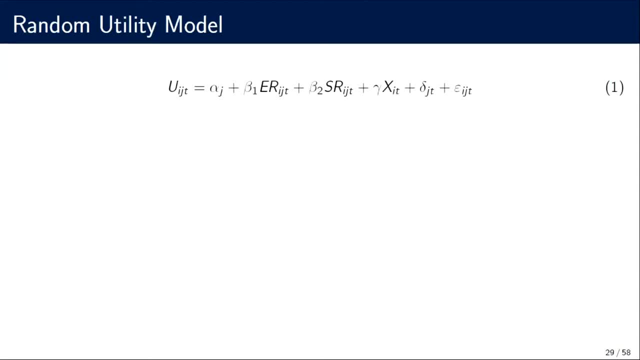 trends of increasing carbon services, so it might give us a suggestion that the policy may have a small effect overall. so we are going to have a discrete choice model, that best that is based on the random utility model. we are going to have a alternate alternative, specific constants for each of the crop practices. so, for example, corn no till, corn reduced till, soybean no. 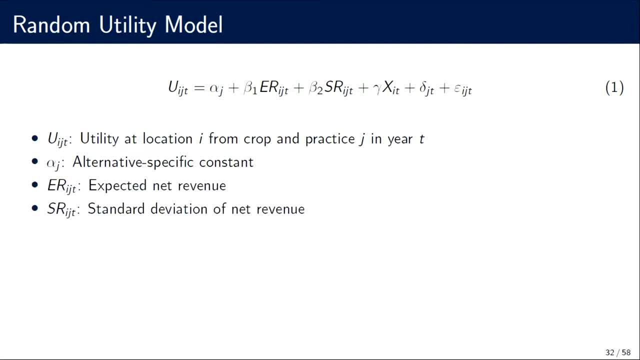 till, etc. and what we are interested in is the average net revenues or profits, and the standard deviation of net revenues. we want to know how they affect the preferences over crop choice for producers. we have other controls as well, like lag crop choice, and we also allow year specific time trends, that their coefficients are crop and practice specific. so 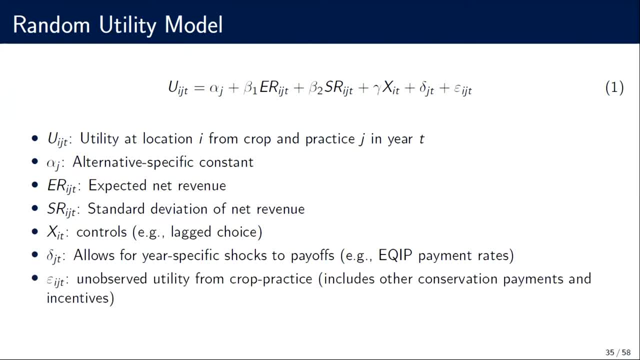 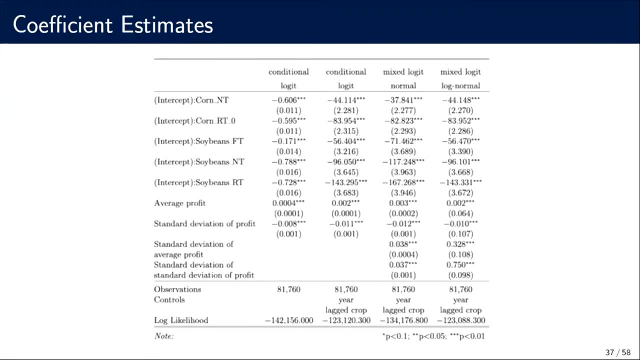 they allow for heterogeneity across crops, the crops and practices. and then we have an unobserved portion of the utility, that we make certain assumptions so that we can represent it as a multinomial logit and mixed multinomial logit model. so i'm going to briefly show the results of the multinomial 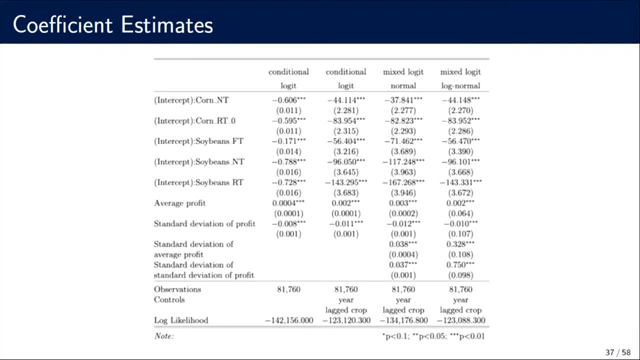 or conditional logit and mixed multinomial logic models, because the results are overall very similar in terms of what they show. i'm going to just briefly mention what this column does. the first column is the conditional logic model without any control. the next column is conditional logic model with controls which include year and crop- a large crop effect- that vary across. 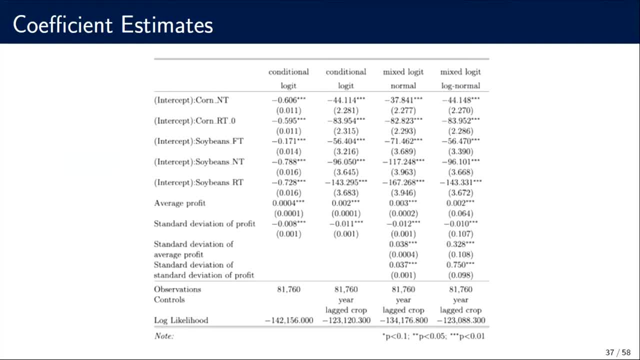 different crops and alternatives and the last two columns are mixed multinomial logic models. in this column we assume that expected profits or net revenues are normally distributed so that we don't impose a specific distribution on that. it doesn't have to be positive, but in the last column 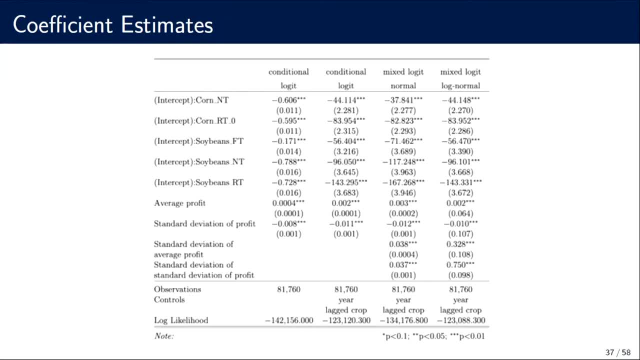 the imposed positive requirement and so the distribution is log normal. so net revenues have to be positive, so we force that in terms of distribution and what we find overall is that utility of the corn full till is higher than the other relative to corn full till. they're all negative, which means 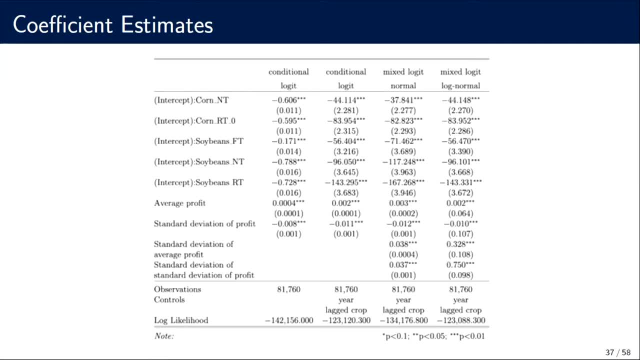 that the profitability of corn full till is higher and it's being selected more often, but also that we find that average profits, as they increase, the utility gets higher and then the crop and practice is more likely to be selected. at the same time, producers don't like variability, and as standard deviations increase, they tend to 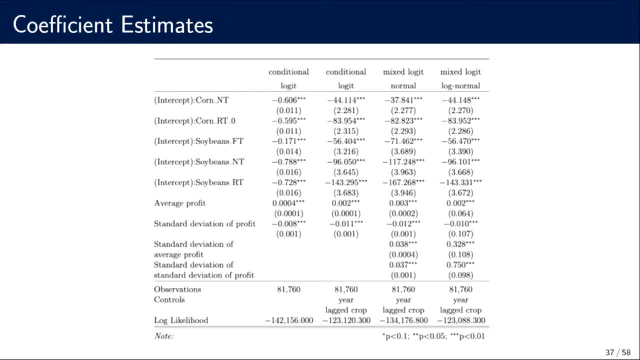 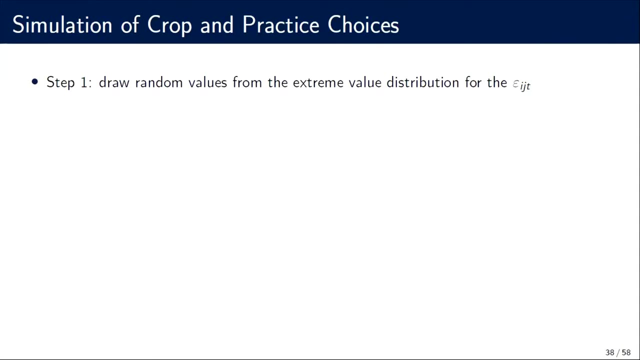 decrease the utility and for selecting a specific crop. and the mixed multinomial logic models show significant heterogeneity in terms of responses to net revenues and standard deviation of net revenues. and then we get these preferences and then we simulate different uh for different prices. we first draw an epsilon term from the unobservable part from the 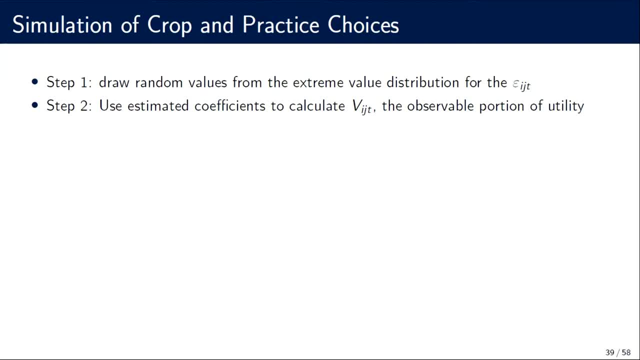 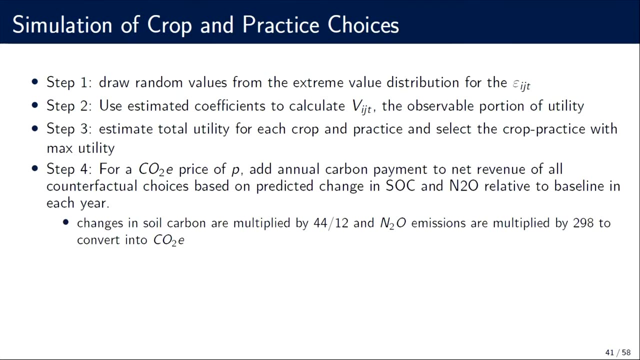 extreme value distribution. we estimate the v hat here based on the coefficients that we estimated and based on the values for each of the points, and then we estimate the total utility. we find the maximum utility and then we simulate for different prices of carbon. basically, we have certain, we have different levels of co2 equivalent prices and we estimate the expected and standard. 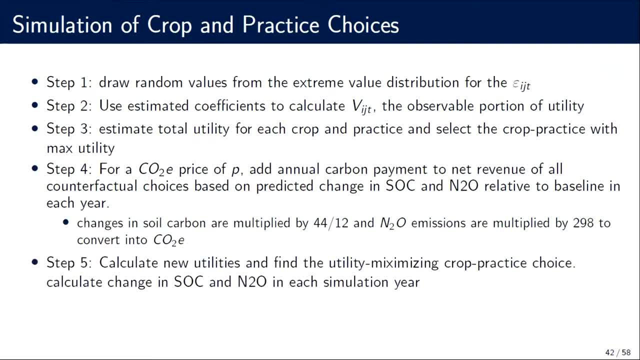 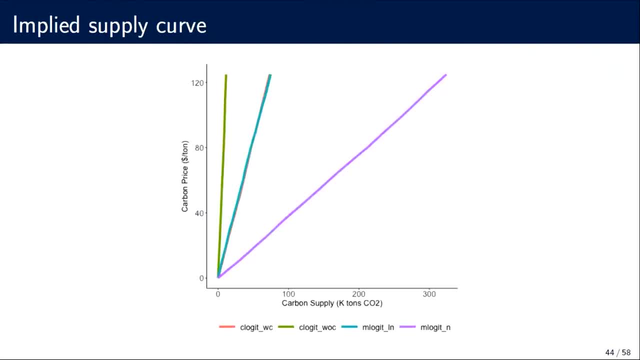 deviation of net revenues. and then we simulate that for those levels, we simulate that for those different prices for and we get the supply curve basic. what we find is that overall, the supply curve can be very different across different practices, across different modeling assumptions. the more heterogeneity we allow, the more elastic it will become and as we include controls, 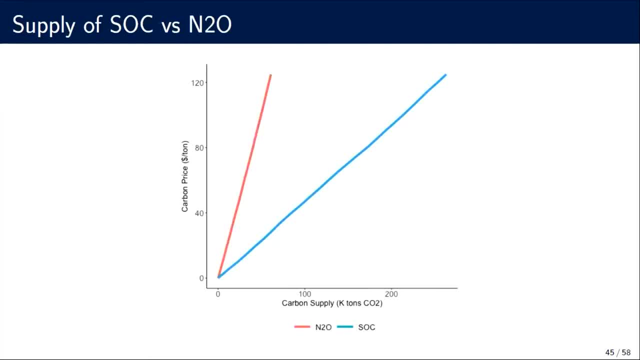 the supply curve tend to be more elastic as well. and then we also see that most of the services come from soil carbon sequestration rather than into reduction in N2O emission for any given level, given price. I'm going to go into my time a little bit. 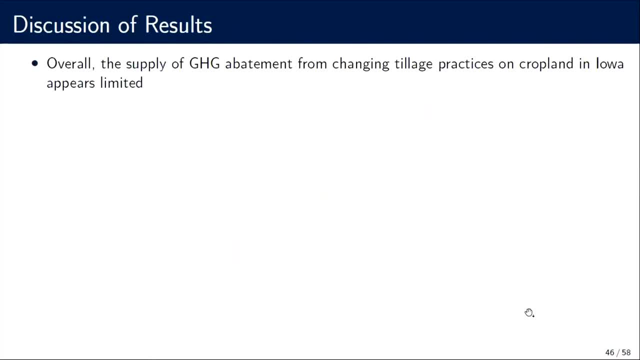 then I can take it from the questions, if that's OK. So what we find overall is that when we compare these results from these supply curves, we find that the scope for a carbon offset market from agricultural production overall is very limited when we think about the volumes that. 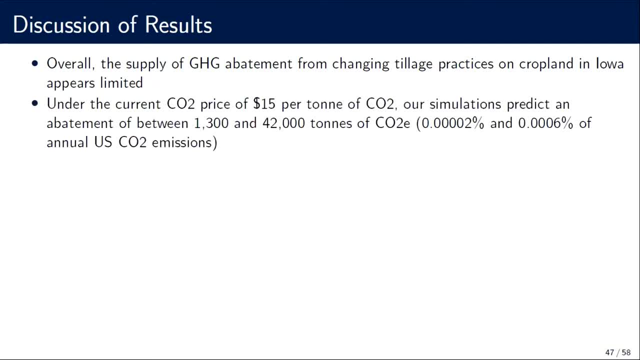 can be sequestered. Let's think about the CO2 equivalent price of $15 per ton. In that case, using the different supply curves that we have, we end up somewhere between 0.00002 and 0.0006% of annual emissions. 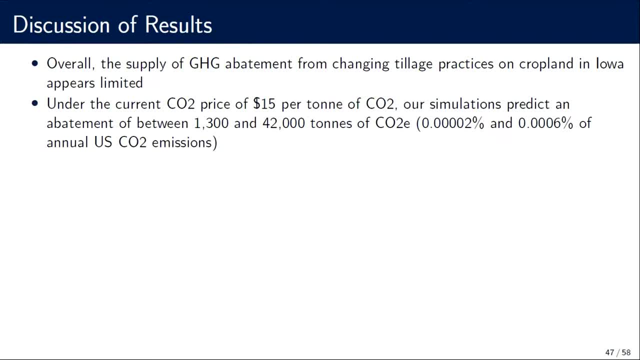 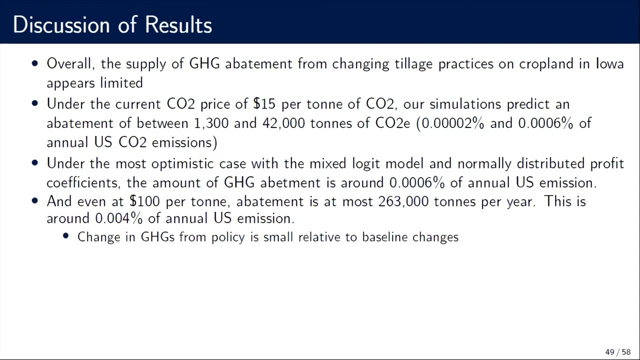 for the entire US, which is a very small percentage of that. In the most optimistic one, that if we think about the mixed multinomial logit model, we end up with 0.0006% of the annual emissions, And even if we assume the price of $100 per ton of CO2. 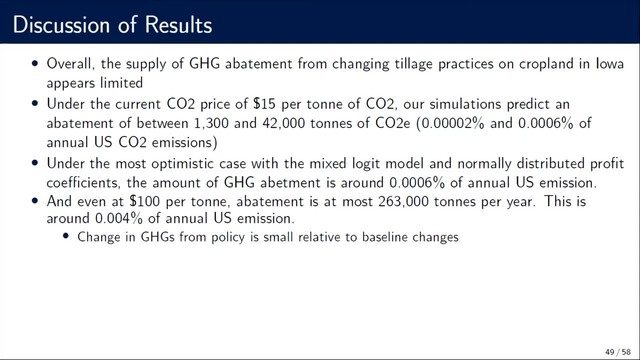 equivalent, we still end up with 0.004% of the annual emissions for the US. So the scope for this carbon offset market is really limited relative to the baseline And what we may think about if we. this is for Iowa and we want to expand this model to the entire US. 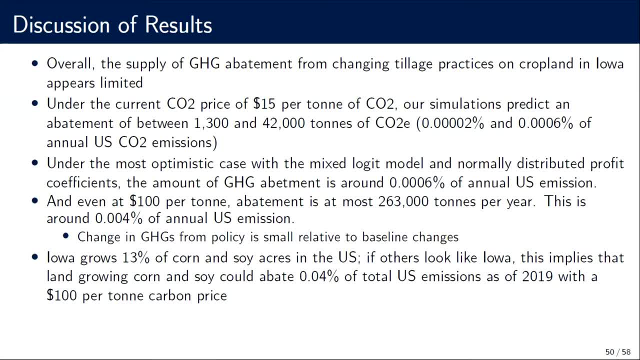 well, Iowa still has a lot of potential compared to the rest of the US. So we're going to have to look at the carbon offset market. So let's look at that. Let's look at that, And if we expand it to the entire US, we end up with somewhere around 0.04% of the annual 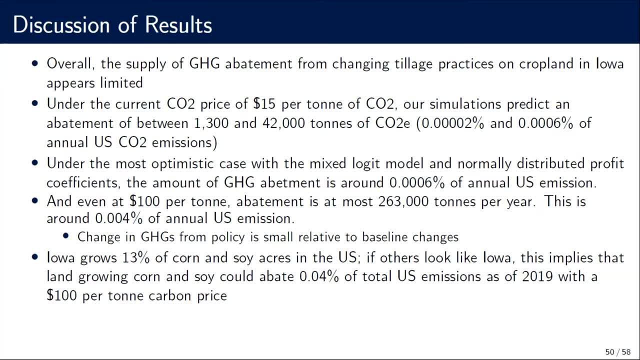 emissions at the price of $100 per ton of CO2 equivalent. So, at the end of the day, the scope for this carbon sequestration market is very limited. Overall, this is part of the tool set that the government or the marketplace can use. 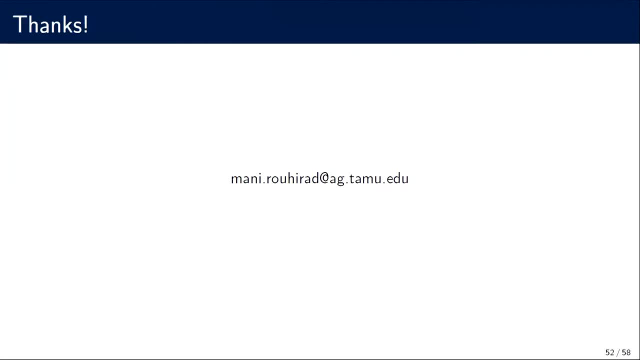 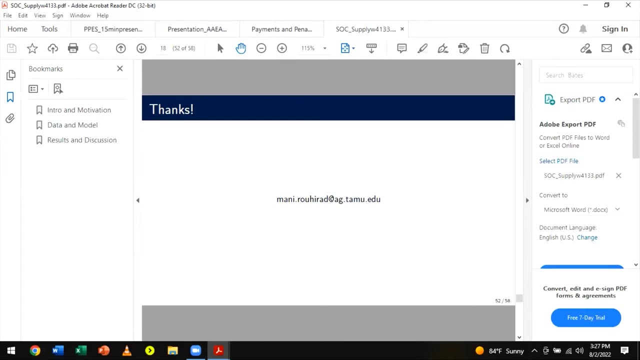 but the scope for it is very limited. Thank you, Yeah, I didn't prepare any slides, sorry. I have one simple thing. Here's the time limitation. I mean Gideon mentioned his next steps to kind of improve their papers. 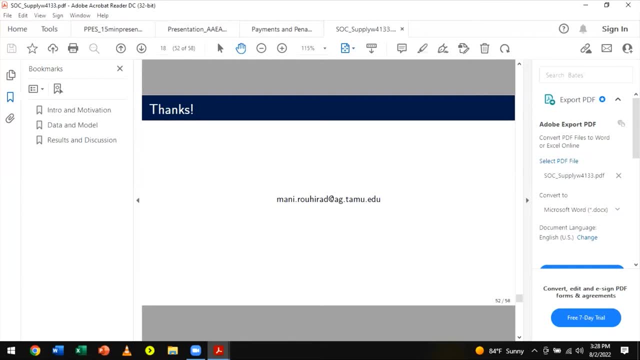 One thing I would like to emphasize is that they use the tillage data. the same use a constant tillage data between the five years, So to improve the accuracy. they mentioned that they may use satellite imagery data. I do see some variations. 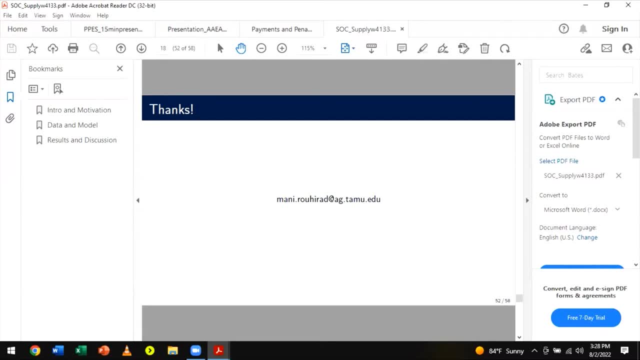 Some variations of the safety adoption between years when I do my study. So that will be very helpful to improve the whole research. Yeah, I think I will just give the simple comments. Any questions? How many Go ahead? So I really like this question. 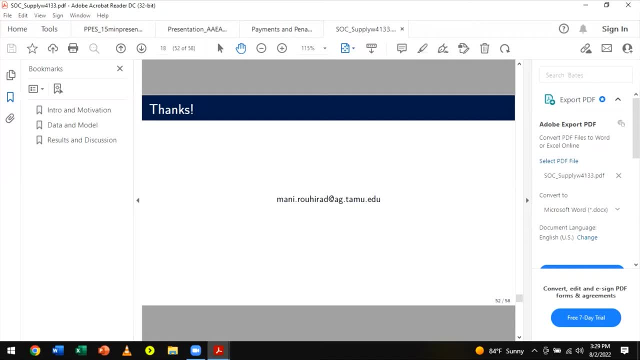 I think it's very important. I do have a question about it. You say it's like location. is that a specific spot, or is it like several kilometers or two kilometers like the area, or is it more so like a spot? 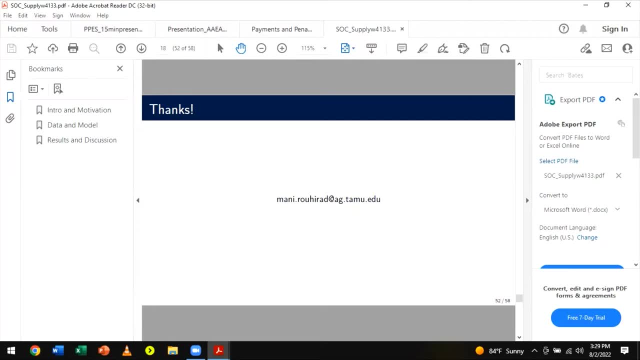 Yeah, that's a really good question. So this is really like a point. I've seen the maps of those NRI points, how they pick it And they have some statistical way to get to those points So they zoom in into the land more and more statistically. 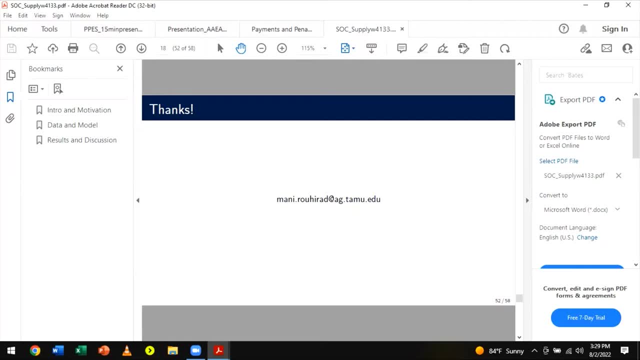 And then they get to a part of land that is kind of zoomed in- I forget what they call this specific- But then they pick an actual point from that point, And this point can be part of a farm, for example, And then that farm will become part of the NRI history. 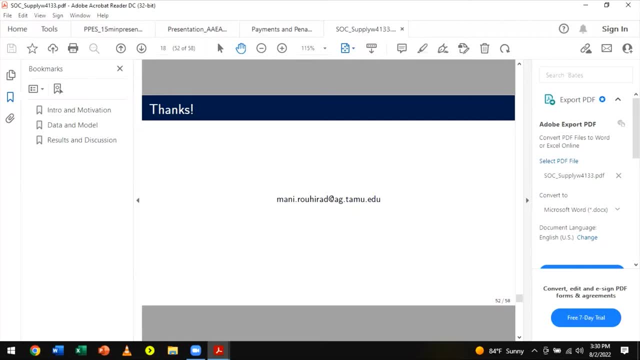 And yeah, so they then collect the data. I think for the entire farm, not just only for that point, But the carbon itself. I think for only that point probably. I was just thinking about the entire farm. Is that part of what happened to it? 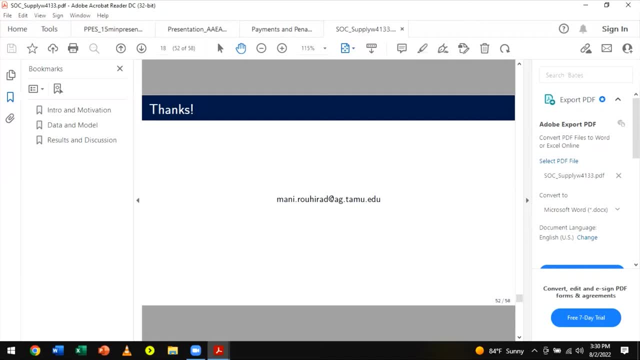 I do think it's not something to the model. Yeah, Yeah, Thank you. Yeah, I think there are things that they just know about the points. Yeah, We struggled a little bit because these points are then representative of the larger area. 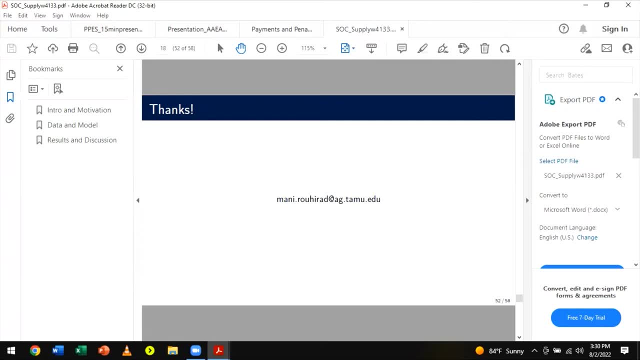 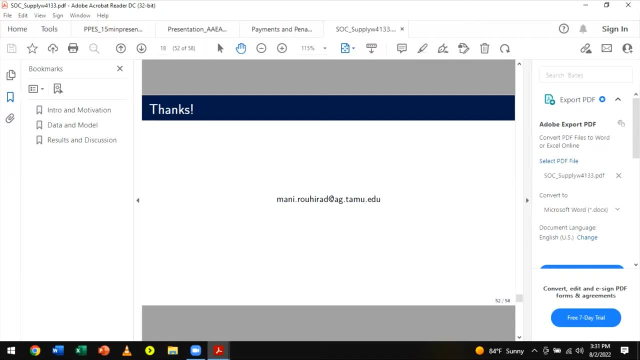 Yeah, Yeah, Yeah, Yeah Yeah. Like I just want to make, Was there any overlap between the two slots? and So I think they tried to, Because those are statistical points that are selected. they want to represent the entire landscape randomly. 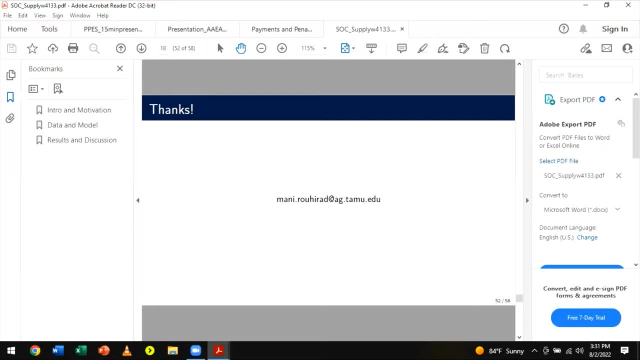 Okay, So they try not to do that, So that there are two points next to each other, At least a few pictures that I've seen how the points were selected and I don't have access to those NRI points. that, where they are, it is part of our. 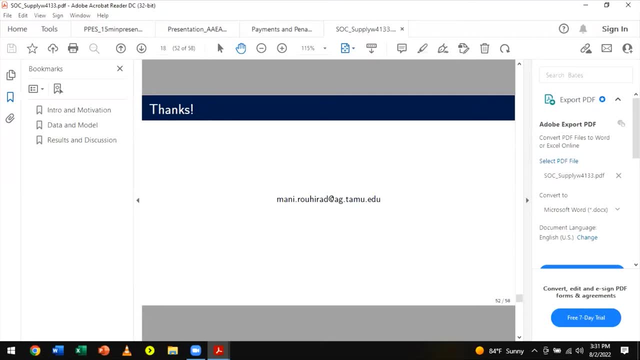 one of our limitations, But the person that has access- they have showed us Steven has access to those and they have showed us how like an NRI point will look like And it sounds like it's just one point, one point in an area. 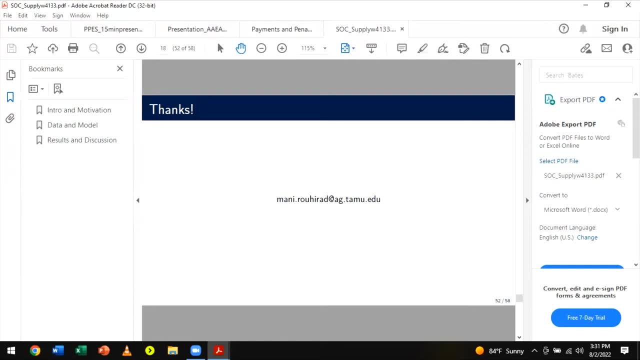 So there are not two points next to each other. that So I don't know if you want something like this. you know because the 28,000 years you know they have 13,053 years here and that's like half of the data that they know. 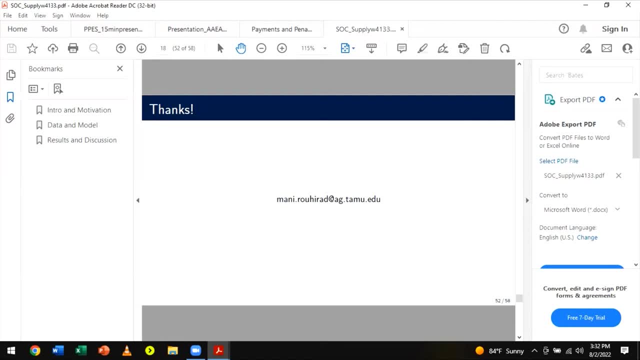 for like they can pick up and do the new data at an annual level, which is good, But also I don't think that information is possible the more you tell, like the college and all the other intelligence companies, So like if you are looking at that. 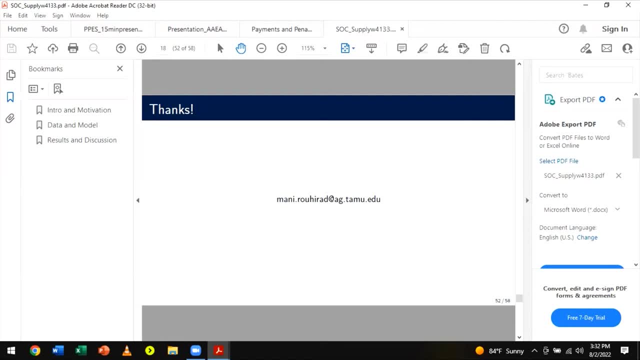 you know, like, if you are looking at that. you know like, if you are looking at that, you know like, if you are looking at that, you can just take a look. Okay, thank you, I don't know how to check. 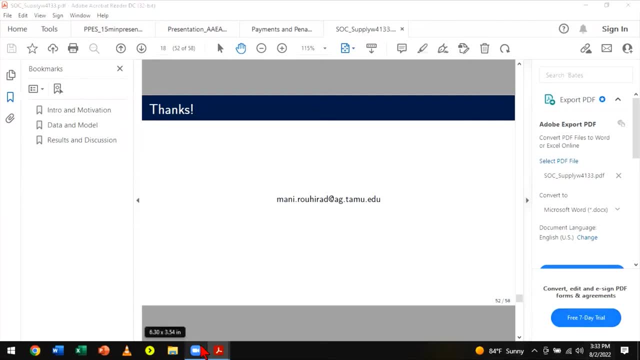 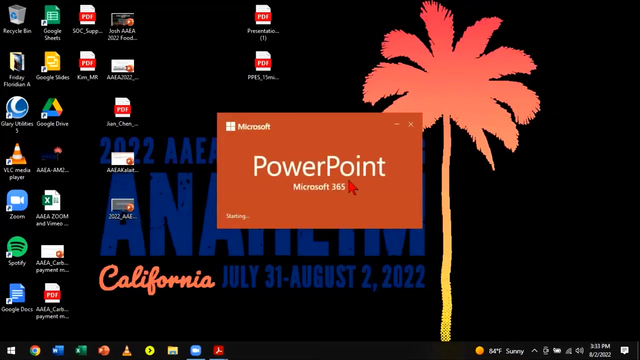 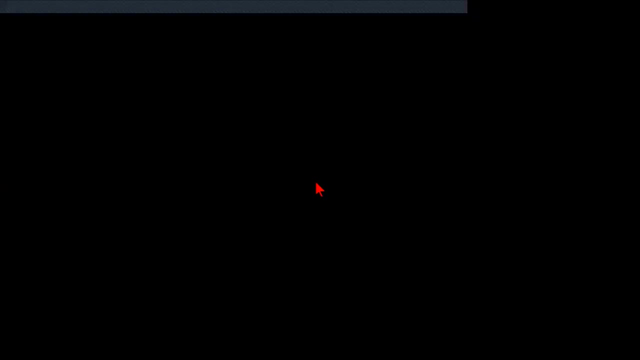 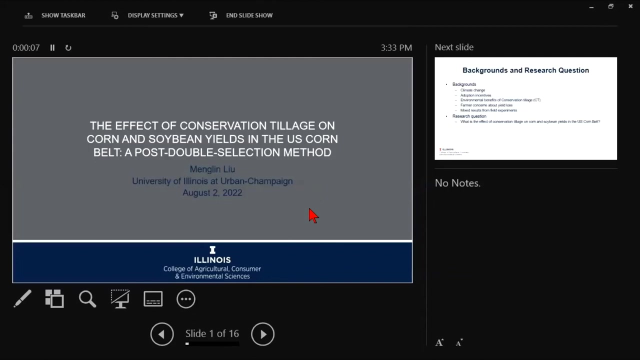 Yes, this was zoom break. Yeah, I forgot to check that for you. Where is the no? no, there's no, there's actually one. Okay, I will get started. My name is Mo Ling Liu. I'm a PhD student at the University of Illinois, at the Abundant Champaign. 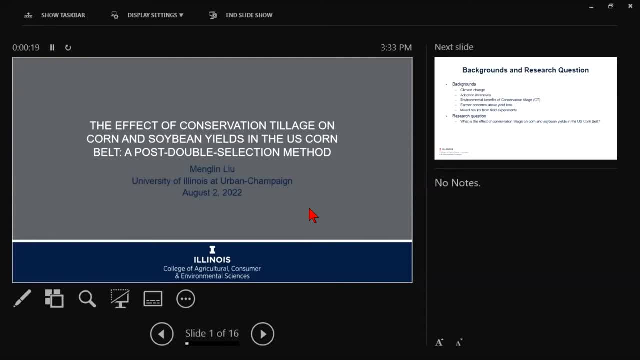 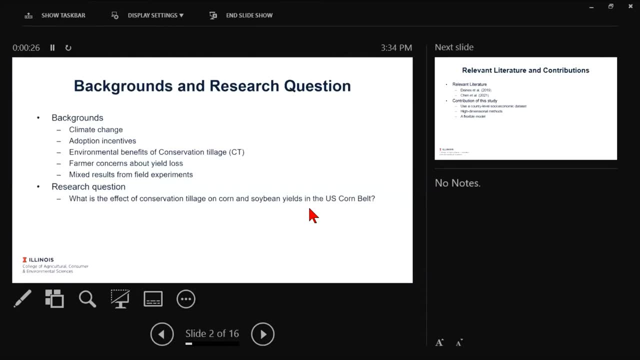 I'm going to talk my paper today. I'm going to talk about the effect of conservation tillage on corn and soybean yields in the US. Corn Belt, a post-double selection method, Also with some backgrounds for this research. the climate is changing. 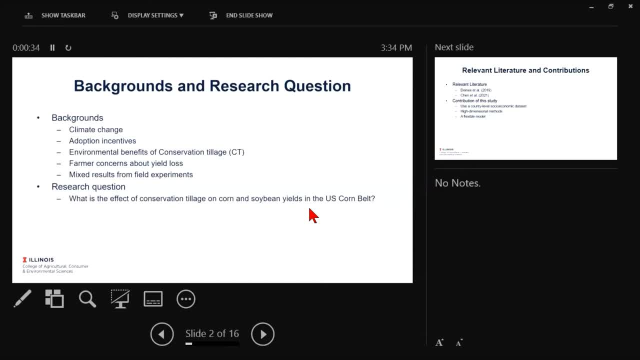 Extreme events are happening more often. The private initiatives in the government are taking actions to promote the adoption of conservation practices that sequester carbon in soils and vegetation. Conservation tillage, as one of those practices, has been recommended for adoption for years due to its environmental benefits. 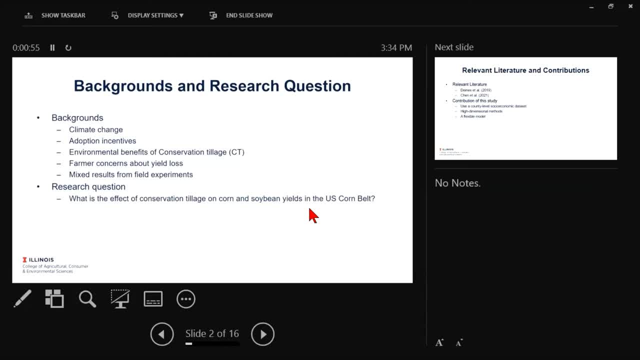 However, farmer concerns about yield loss might be an impediment to expanding its adoption. Many studies have been done, based on field experiments, for assessing the yield effect of CT. The results are mixed due to variations in locations, weather and soil conditions. To get a more generalized result, I'm interested in using the observational data to find the average effect of conservation tillage on corn and soybean yields in the US Corn Belt. 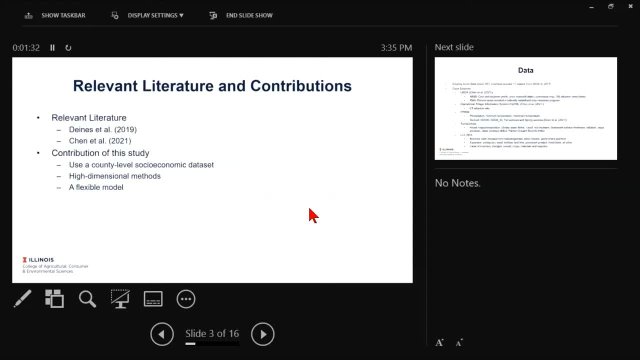 There are only a few observational studies have been done on this topic, The two most recent ones Danis et al 2019 and Qing et al 2021.. Both of the studies used satellite imagery data for CT adoption. Danis et al 2019 applied causal forest to field-level data without including any socio-economic variables. 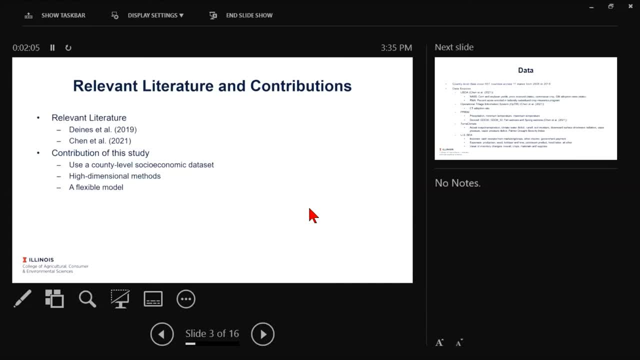 While Qing et al 2021 used a linear fixed-effect model on county-level data, including a few national and state-level socio-economic variables, They found similar results. CT adoption has no negative effect on corn and soybean yields. However, both studies have some limitations. 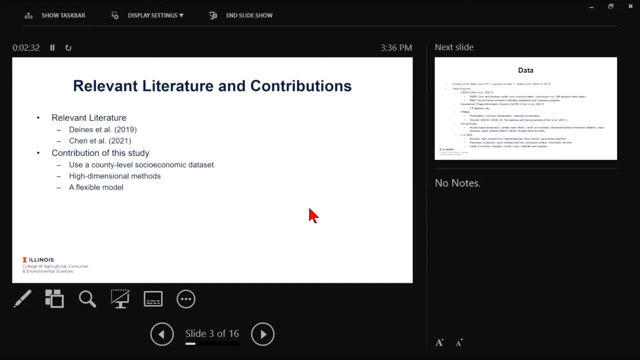 One of the concerns is omitted: variable bias. If the socio-economic variables that impact both yield and CT adoption at the same time, they may cause some issues. They may cause some issues. Besides, the linear specification used in Qing et al 2021 might not be the correct one, since the order of CT might be influenced by the quadratic terms or other nonlinear form. 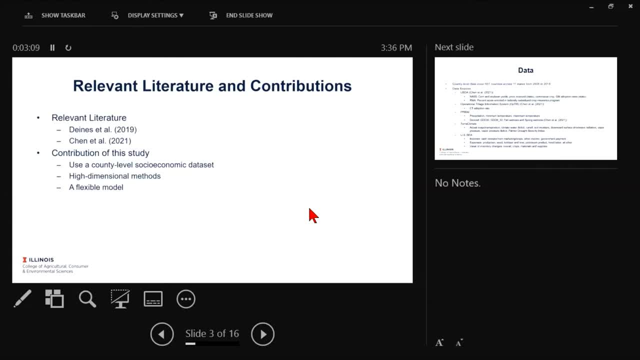 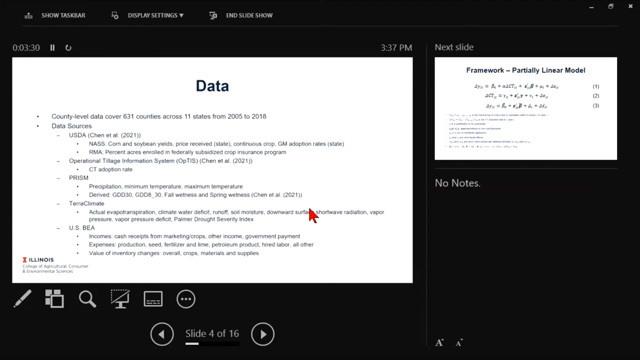 To address those issues, I used a county-level socioeconomic dataset and applied high-dimensional methods to my model and apply high-dimensional measures to a more flexible model that allows the nonlinear chain to interact with county-level time-routing characteristics. The county-level data I used covered 631 counties across 11 states from 2005 to 2018.. 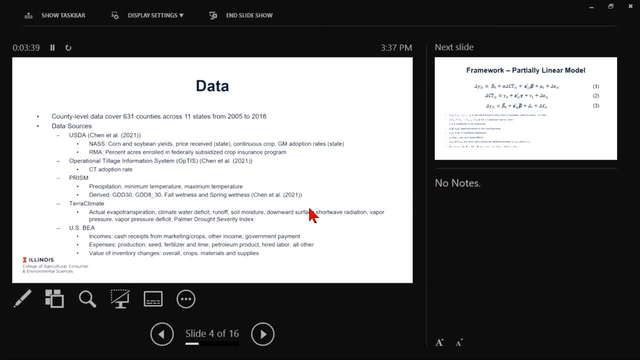 I used some of the data I used in China, Adult 2021, such as corn sowing yields, state adoption rates, crop rotation rates, crop insurance rates, state-level price received and GM adoption rates and fall wetness and spring wetness. 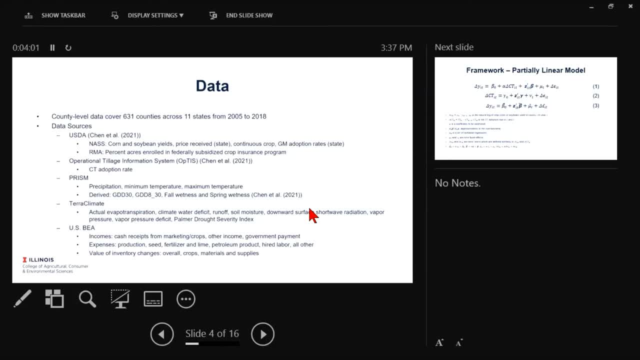 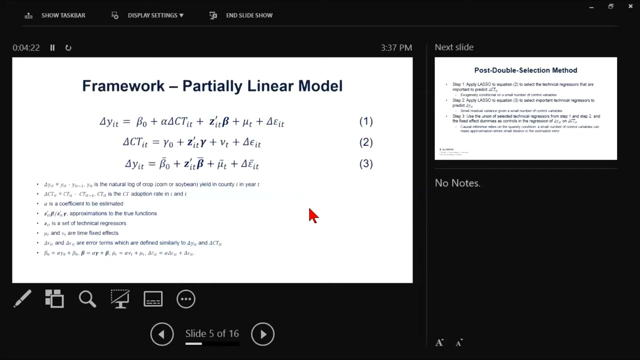 In addition to their data, I calculated county-level weighted average of some weather and climate variables. The county-level socioeconomic data I used in this study, such as incomes, expenses, and evaluate inventory changes from USDA. I'd like to talk a little bit about my framework. 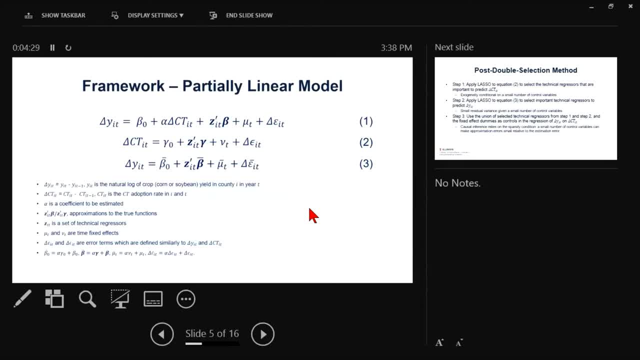 Equations 1 and 2, constructed following partial linear models. Delta Yt is the difference of log of the yield in count, Kommett and Yt. Delta Yt is the difference of log of the yield. Delta Yt is the difference of log of the yield in count, Kommett and Yt. 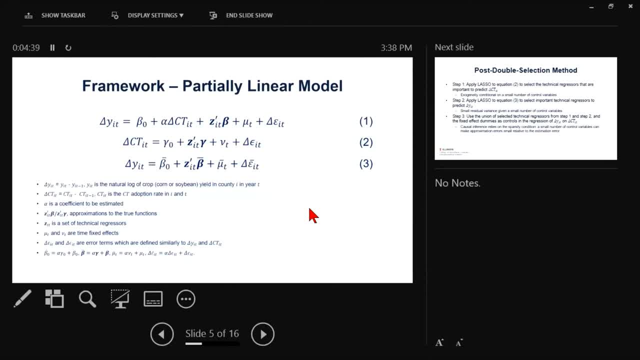 in year t. delta ct i t: the difference of the ct adoption rate in county i in year t. The first difference structure helped me to control the time-inward characteristics. Z i t prime beta and Z i t prime gamma are approximations to the true functions. 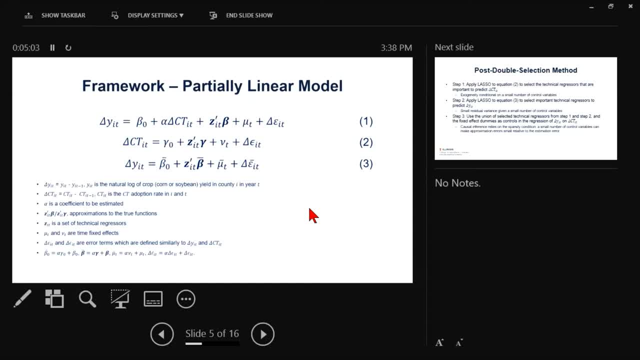 An important assumption here to make the variable selection method, which I will talk about later, valid is the sparsity condition. Sparsity condition means that only a small number of non-zero coefficients in beta and gamma can make the approximation arrows small relative to the estimation arrow. Z i, t, the set of technical regressors made up of the differences. 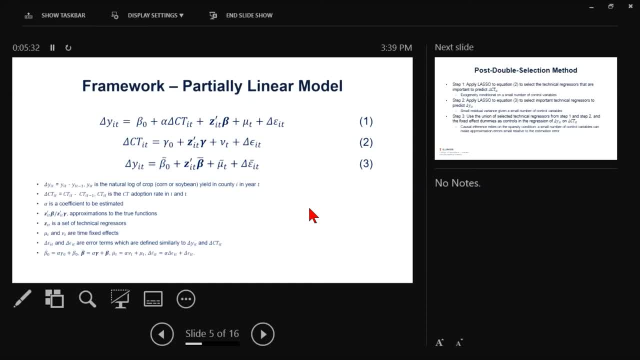 and lags of weather and socioeconomic variables. The initial levels and the initial differences of weather and the socioeconomic variables and the ct adoption rates. the quadratic terms of the preceding variables, the interactions between the differences and the interactions between all of the variables with time t and t squared, This set of variables 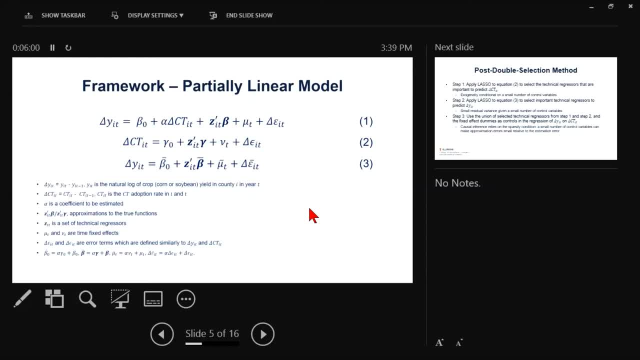 corresponds to a cubic trend for the level of yield and ct adoption. that is allowed to depend on county level of time varying characteristics. v i, t and v i t- here is the time fixed effect, which capture the national aggregated time trend. Equations three: here is a reduced form. corresponds to equation one. 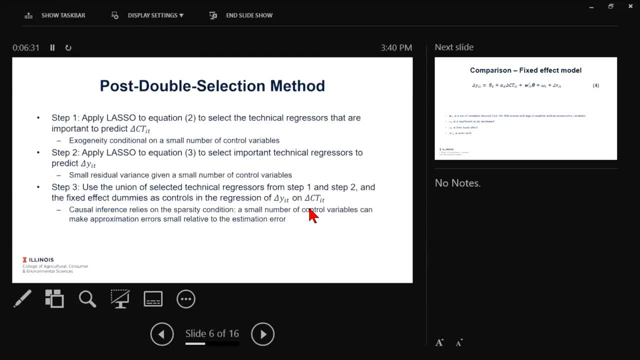 After the model is constructed, I apply the post double selection method to find the causal effectiveness t on yields B. Step one: I apply LASSO to equation two to select important and confounding factors. Step three: I apply LASSO to equation three to select important factors. 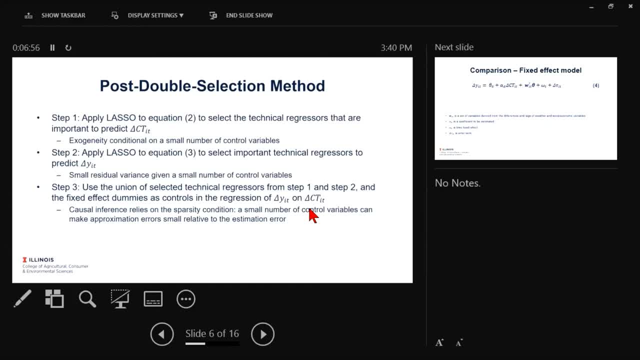 to make sure the residual variance is small. In the final step I used the unit of the selected technical regressors for these three factors as reference factors from step one to step two and the fixed effect dummies as controls in the OIS regression of. 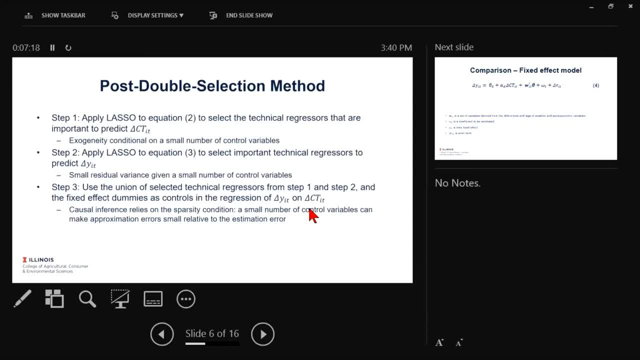 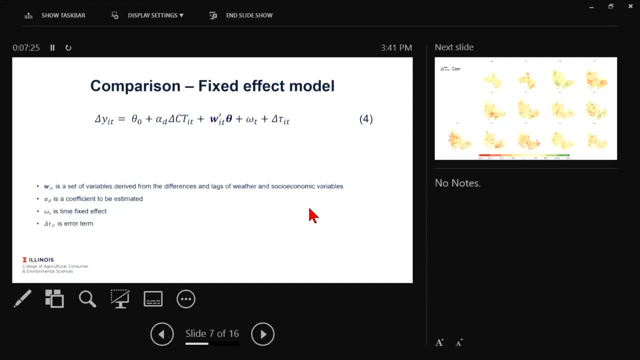 delta y, t on delta c, t, i, t. This causal inference relies on the specific condition I mentioned earlier. To examine the double selection estimator, the performance of the double selection estimator, I also specified a linear fixed effect model, WIT. here is a set of variables derived from the differences and lengths of the weather. 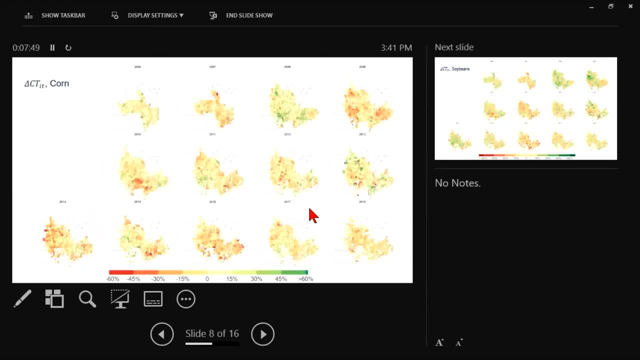 and socioeconomic variables. Before I jump into the results, I'd like to show you the variations of the difference of the C? t for corn and soybeans that are captured by the data, The overall. the overall variations for for the difference of safety for corn is from the negative 16 percent. 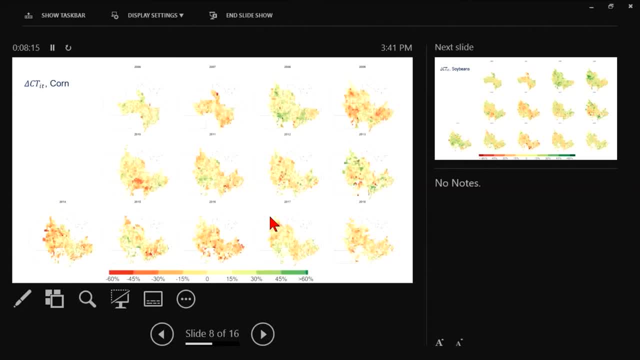 60, 60 percent to positive 60 percent, Most of the uh, most of the variations between negative 15 percent to uh to positive 15 percent. Some of them may be up to um negative 30 percent to 30 percent. We can see the. 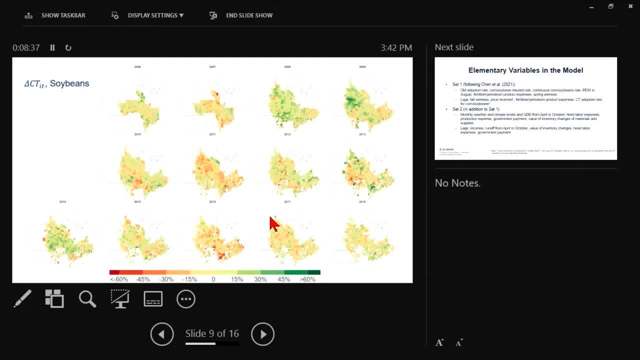 the difference between the. if you have a forwardaren the, then you you 59 percent to positive one for th świ it and then you one. the negative set units of your life, Merkin and t and et. Among them is the difference between肅 being in the KST. 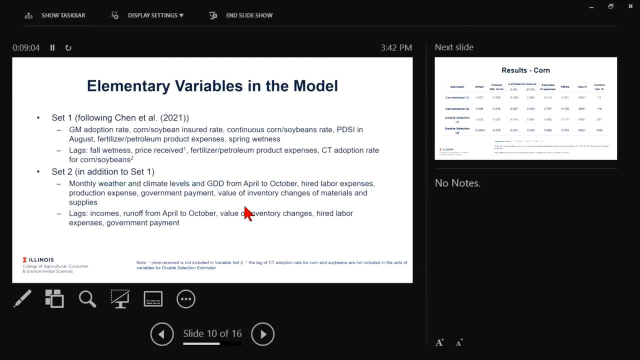 on th rr and because I did not Shiva, but it was part of that study- The major difference between China and the Umi così ni variables. in the two specifications I mentioned earlier I followed 10.0.2031 to determine the first set of variables, but I replaced some of the variables used in their study. 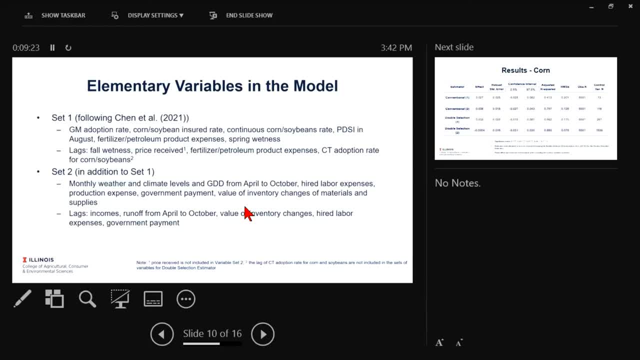 I used the PDSI levels instead of the PDSI dummies to capture the year-to-year variations. I use the fertilizer and fuel expenses- the county level instead of the national level. fertilizer or fuel prices Based on the variables in the first set, I add some monthly weather. 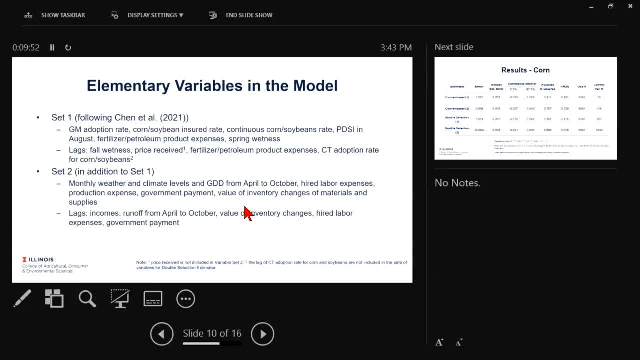 and climate levels and GDD. from April to October. hired labor expenses, production expenses, government value of inventory changes of materials and supplies and the lags of income runoff. from April to October: value of inventory changes, high labor expenses and government payment. 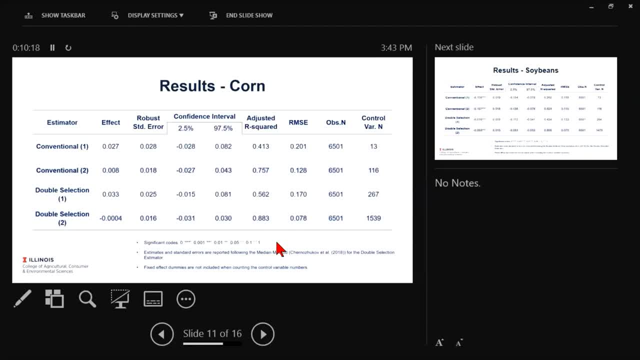 Here's some results for corn. In the first column, the conventional means using the linear fixed effect model. Double selection means using the post double selection estimator. One. two represents the first set of variables and the second set of variables The effect and the robustness standard arrow reported. 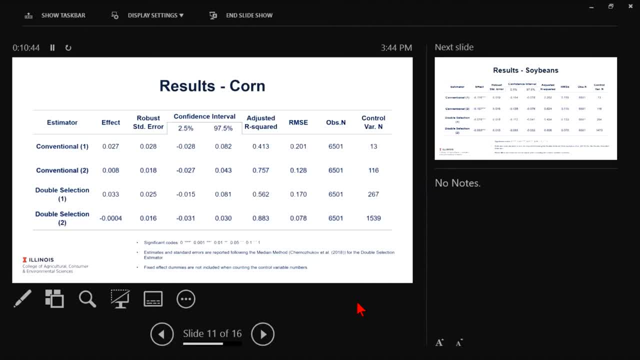 following the median method used in Chernodukov et al 2018.. The effects of the CET adoption on corn consisted across models and the variables used. There's no significant effect of the CET adoption of corn. The model performance pretty similar for corn and soybeans. 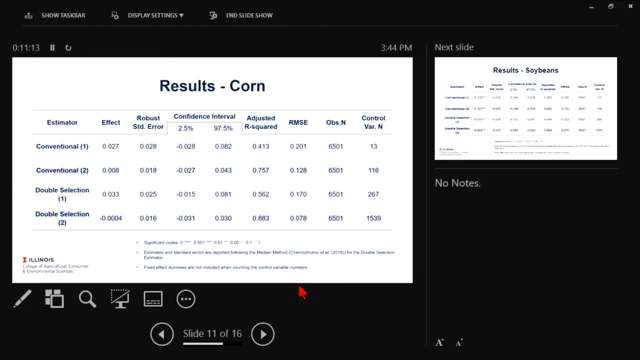 So I mainly discuss the model of performance in the results of soybeans For the effects of the CET on soybeans. they are also consistent across models And the variables used. I find a negative, significant and negative effects of CET on soybeans. 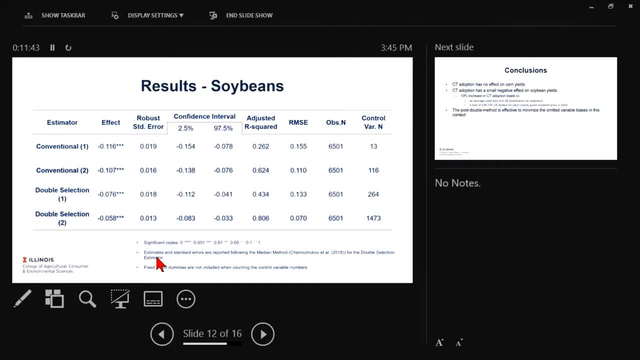 And both double selection estimators work perform better compared to the conventional estimator when using the same set of variables. The double selection process for the first set of variables selected 264 variables out of 270 variables, which means most of the variables in the model. 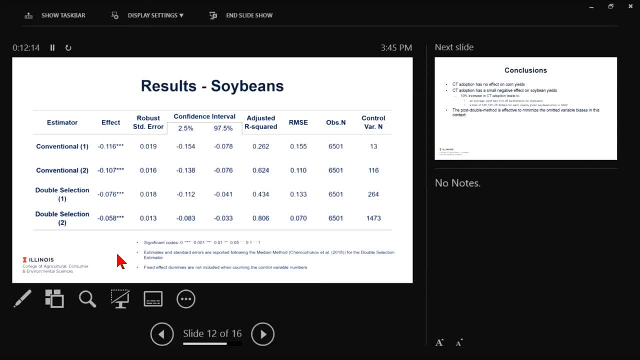 are important to predict the delta YIT or delta CTIT. This suggests a potential omitted variable bias: Double selection. for the second set of variables, CET Selected about 1500 variables out of more than 14,000 variables. Most of the variables selected are the interactions. 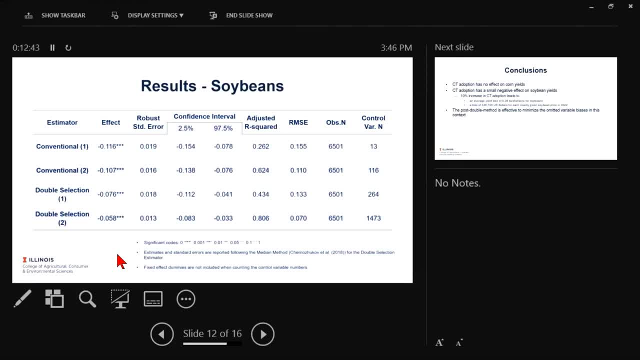 between the weather and socioeconomic variables. All the ways are without interacting with time T or time T squared. This set of variables selected, represent: suggest. this set of variables selected, represent: suggest. this set of variables selected, represent: suggest: suggest. a nonlinear trend depends on a county level. 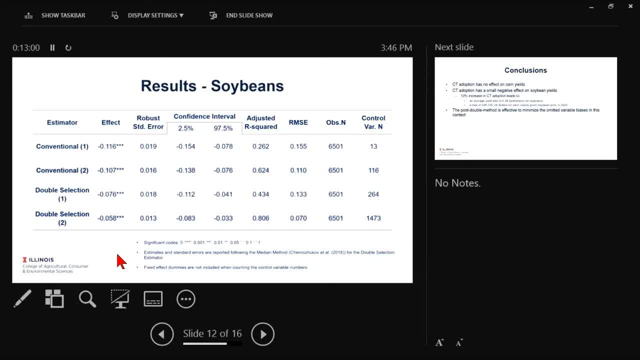 a nonlinear trend depends on a county level time-waring characteristics. Double Selection Estimator Two perform the best. if we look at the robustness arrow confidence interval and the RMSE, The coefficient of this estimator can be interpreted as 10%. If we look at the robustness arrow confidence interval and the RMSE, the coefficient of this estimator can be interpreted as 10%. 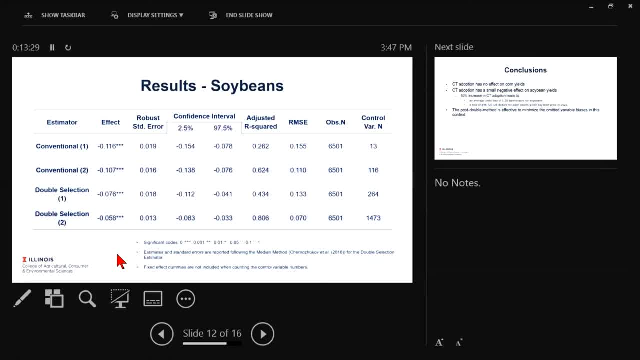 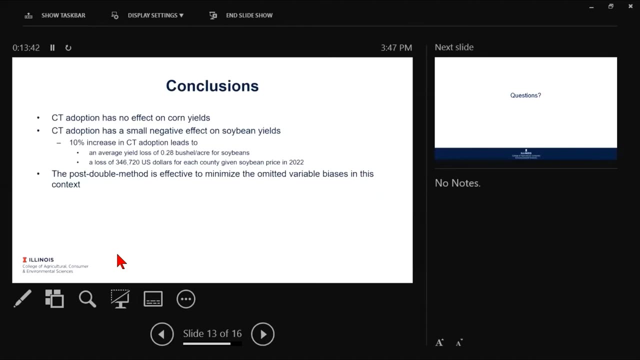 Increase in CT adoption leads to about a half percent decrease in soybean yields. I will conclude my presentation with several key findings. CT adoption has no effect on corn and soybean yields. CT adoption has a very small and active effect on soybean yields. 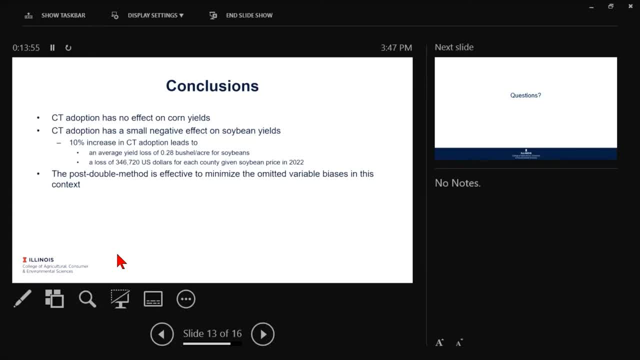 10% increase in CT adoption leads to an average yield loss of 0.28 bushels per acre for soybeans. This can be translated to a loss of about 350,000 US dollars for each county, given soybean yields in 2022.. 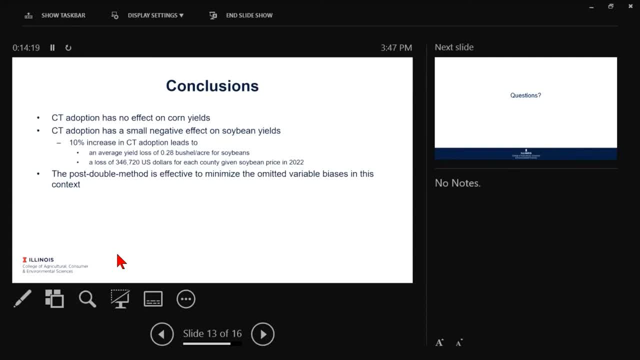 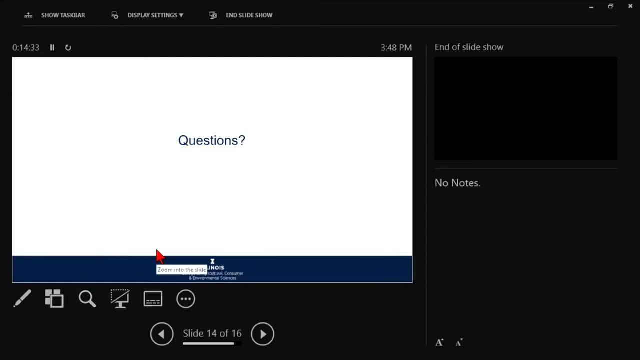 Based on the model performance. the post-double selection measure seems effective to minimize the omitted variable bias in this context. This is the conclusion, Thank you. Thank you, Yes, I have. This is not a well polished paper. Any question or comments? 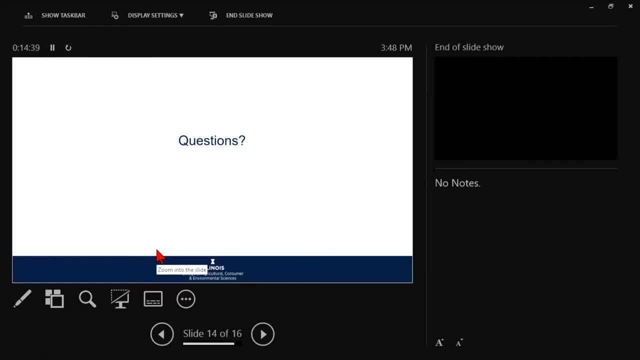 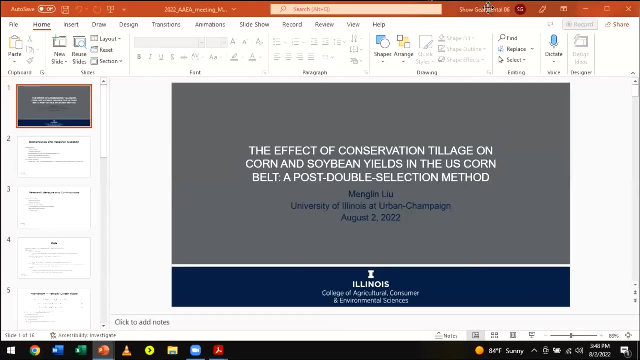 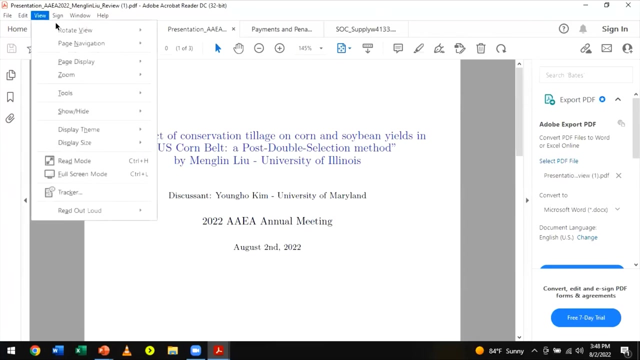 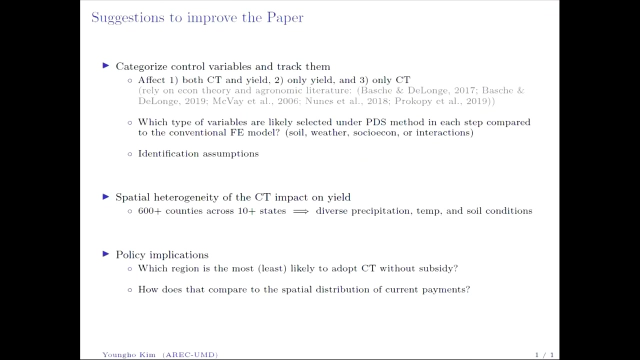 Really appreciate it. But how you for my discussion? Sorry, Let me check if anyone has a question in chat. Yeah, Okay, so I'm gonna briefly talk about suggestions to improve the analysis of the paper. So I have three main suggestions. So first thing is there are, you know, you have a bunch of 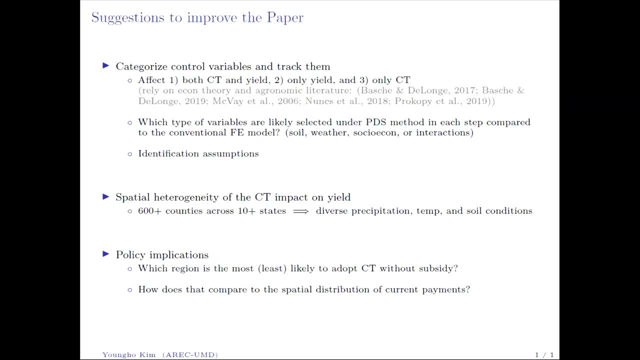 control variables right in the analysis And in the main result table. the number of controls goes from like 100 to like 1500 or like so. additional like thousand or more than thousand variables are included in the analysis And I just want to you know it will be more helpful to. 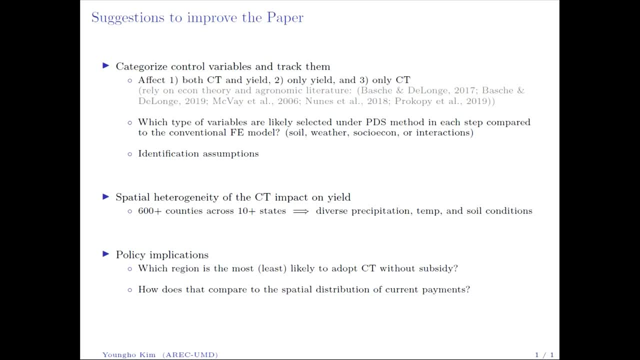 categorize these control variables into three different types. You know, one affects both outcome and conservation, tillage, adoption and ill, which will be confounding factors, And the second one will be controls that only affects ill. So that's going to increase precision of. 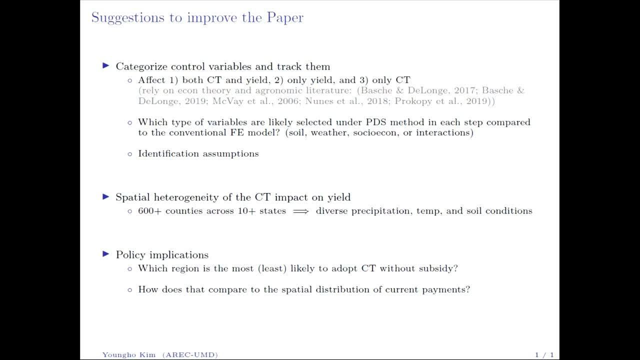 the estimates in the model And the third one is the variables. that only affects conservation tillage And think about which type of, which group of variables are likely to be selected under post double selection method versus, you know, in the conventional fixed effects model, will inform us to think about where the estimate change is coming from. 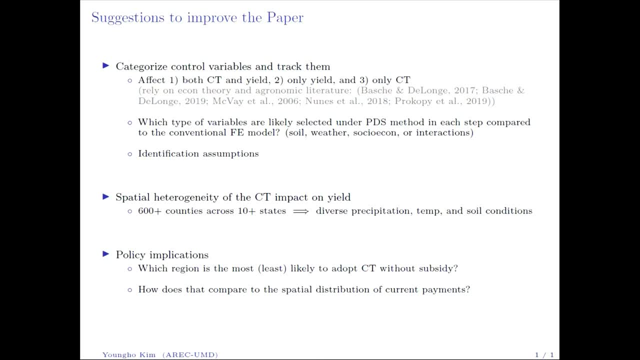 right. So the bias reduction is where the we can think about sign of the bias and where that reduction is coming from, And you can also think about which type of- I mean what kind of variables are included in the in each group, For example. mainly 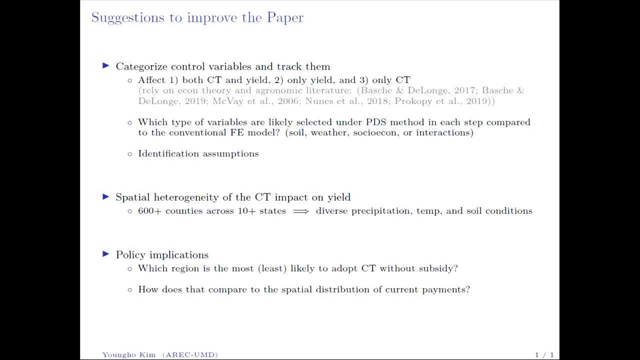 factors will be soil variables or weather variables. Knowing those, breaking down the total number of controls into these three different groups and information on variables that are included in each group will be helpful, And then we can think about identification assumptions for causal estimates. So you know. 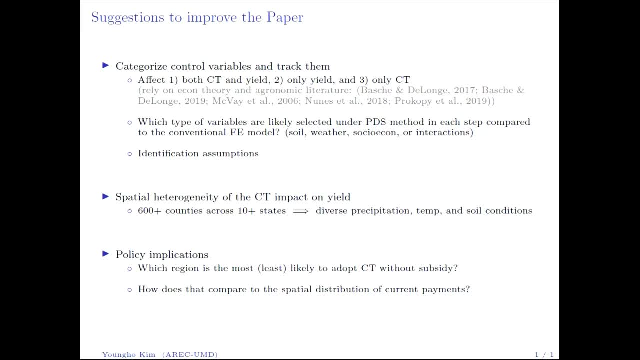 this, this increase in precision of the estimates, and and causal causal estimates are are whether or not. whether or not the estimates are causal is a little different concept. So so I think this will be helpful. And the next, next suggestion is: you know, 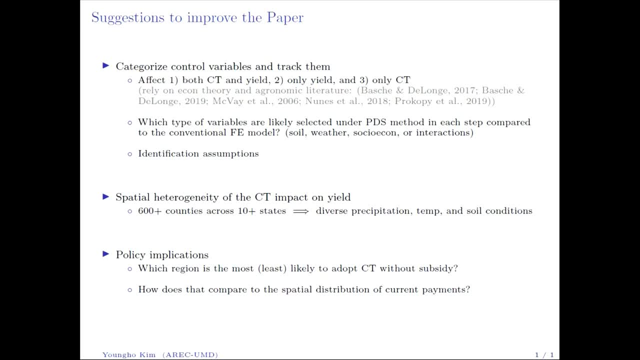 one of the motivation of this paper was to overcome limited externality of the field experiment. So I I just wonder if you can explore spatial heterogeneity of the treatment effect, because you have more than 600 counties across 12 states in Corn Belt region. 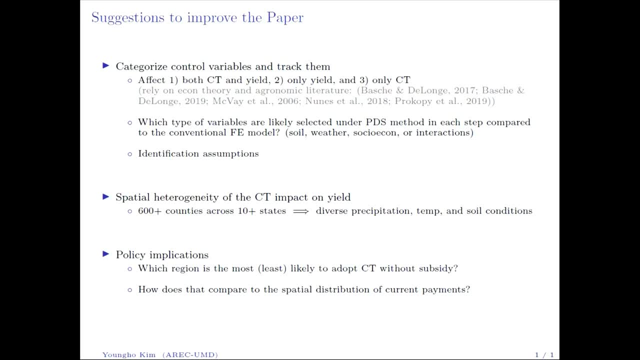 So they will have different soil types, precipitation and weather within the region. So I think one thing you can do is explore this heterogeneity And based on that you can talk about. you know Paul's implication of the analysis, which is now you can think about which region is the most likely or least likely to adopt conservation tillage without subsidy right. 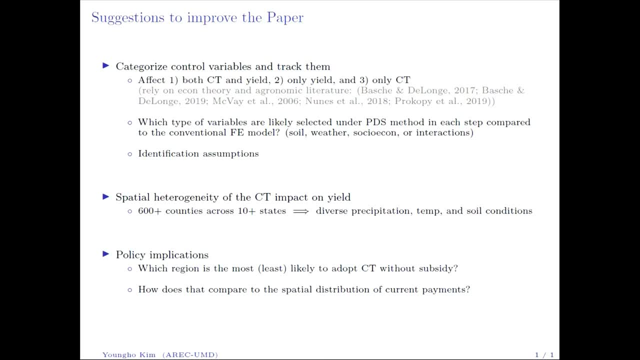 Just based on impact on yield could be a little too much. but because, like you, can also think about crop return, You have all the information: production expenses, fertilizer usage and pesticides and so on, higher labor expenses. but I guess that those information is at the county level, not by crop type. 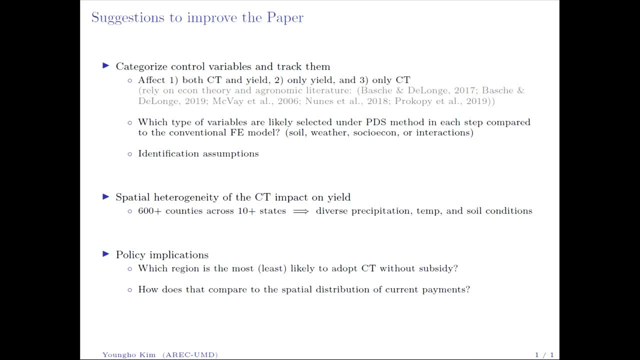 So here what I'm sharing my thoughts on you know. maybe you can answer. you can have answer on which region is the most likely To adopt these conservation tillage without subsidy. Then you know, how does that compare to current spatial distribution of payments, government payments for conservation tillage. 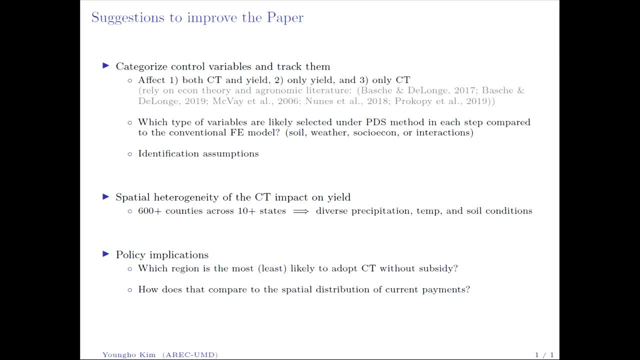 And just this exercise will connect your paper to broader literature on additionality or optimal allocation of government payment on these conservation policies. So those are all I have. I don't know if this ismasıam, but I do have a couple of questions that I wanted to ask you in relation to this, but I think it's a good time to to to ask. 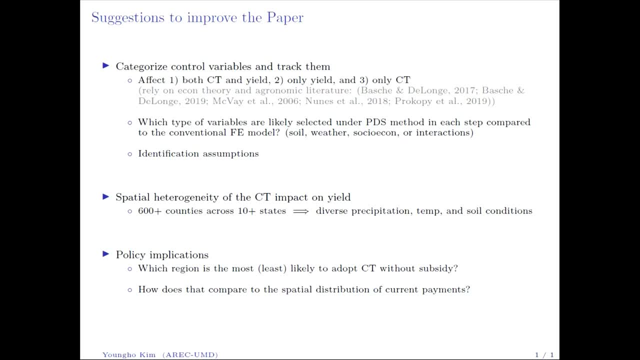 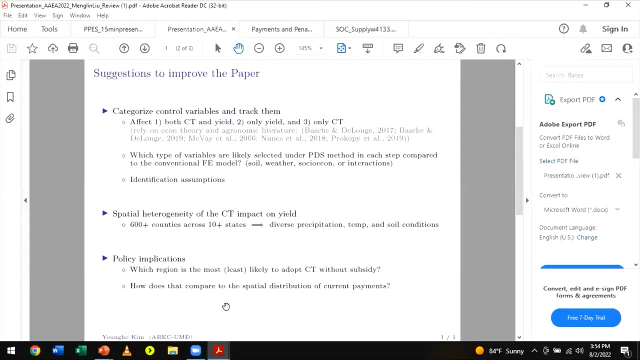 Are there other questions from the audience? I'm just wondering because, like all the, I'm really controlled for They. They didn't work. five Bye, Bye, Bye, Bye, Bye, Bye, Bye. I don't know. I think it totally makes sense, like what other variables you want to actually 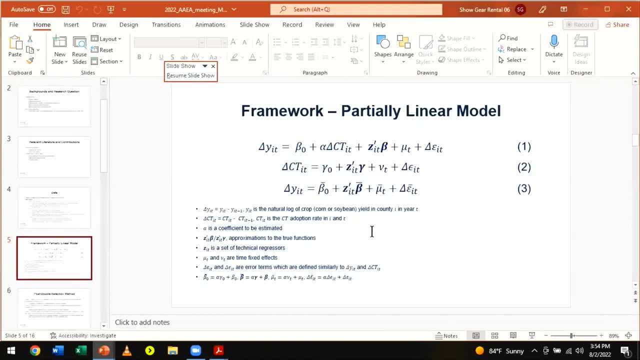 I guess, tell you what you have to do. I don't know. I mean, I think like I think that would be. it's basically like a fixed-effect model. Maybe just try it out and see where what could potentially be different from your model and also the effects from a fixed-effect model. 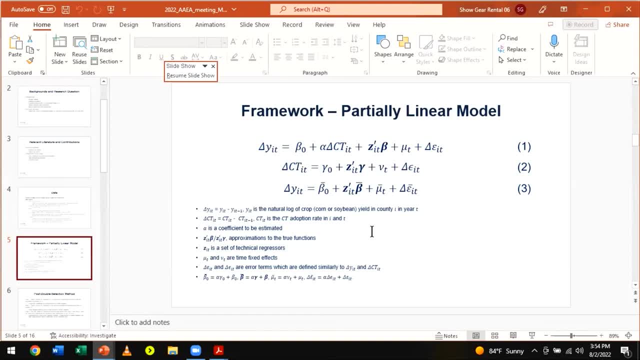 And also, well, I guess we haven't talked about that, Have you already? Yeah, thank you for your comments. Actually, this model includes the county fixed-effect, The first difference. yeah, I use the first difference here. first difference of the yield, the log of the yield and first difference of the CT. 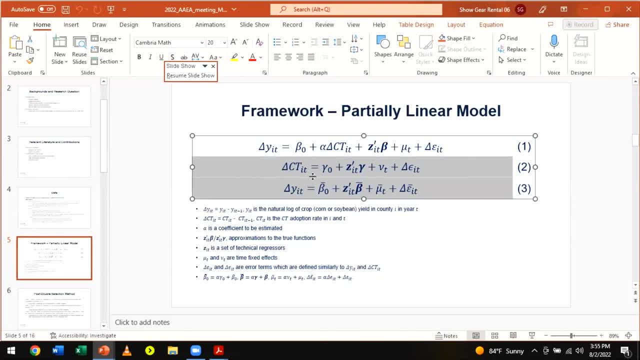 So it's already controlled the time-inward characteristics, So you already controlled the quantity level of fixed-effect. Yes, Oh, okay, sorry, I didn't mean to interrupt your discussion. I was just saying because like, the verb result basically suggests that like conservation and tillage is not like it's, like it's not very significant for formative, significant decreasing, like soil use. 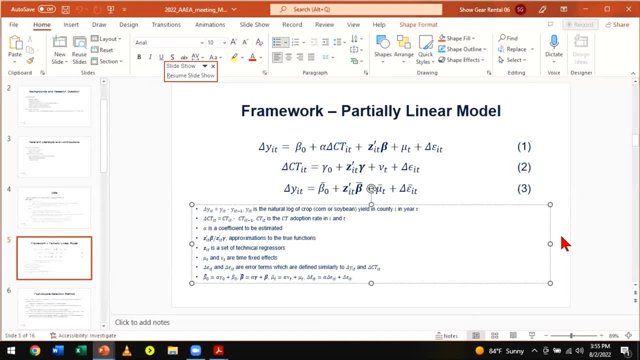 Like maybe I was just thinking about maybe, like it's actually decreasing yield, It could potentially still be made while we're there. in that climate for the society. I'm just thinking maybe it's like worse, considering like environmental benefits. 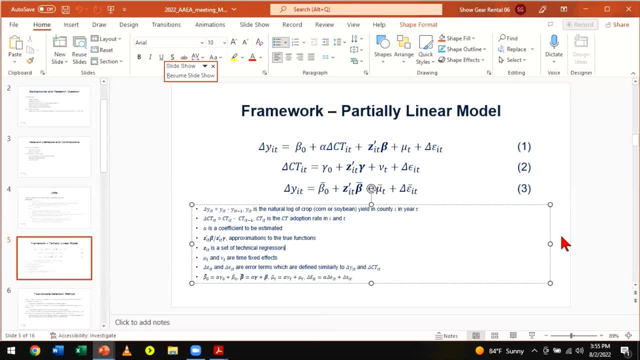 It could be some like benefits where well diversity benefits from, like the tillage, like practice itself. I mean it's making sense that like maybe it's like increasing crop yield for sure, But also like makes the story like more, I guess, like comprehensive, and also like adding a little bit of environmental component to it. 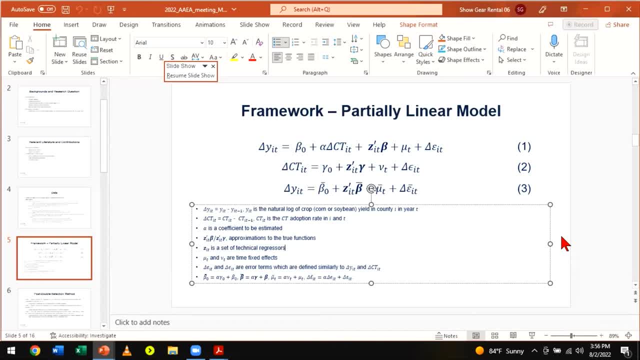 Also considering like the environmental benefit, Okay, Next one. So it's not like a conversation about like the tillage conversion is not everything above the program, It's like a conservation right, It's a conservation program. 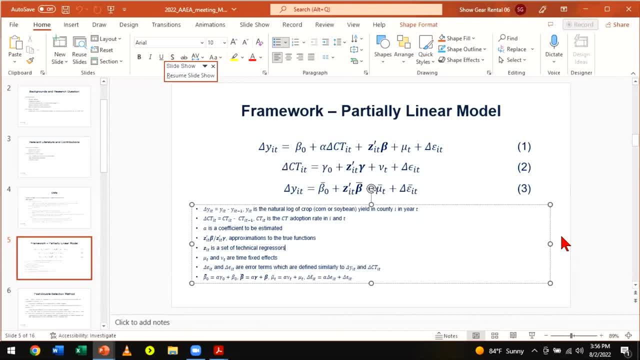 It's very hard to just put it aside and only consider it the effect on you, But I think it's just like I guess future work. If you have like I guess future work you want to work on, it might be a good start if you consider like annual environmental benefits. 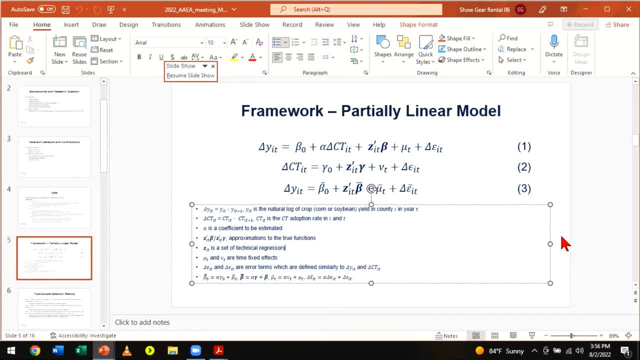 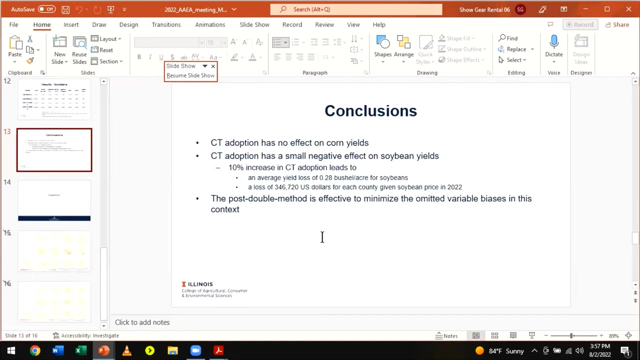 yeah, thank you. thank you very much for your comments. oh go ahead. sorry, uh, constitution, why my slice is not showing here. okay, can i repeat your last sentence? sorry, yes, yes, yeah, definitely, i mentioned that in my paper. yes, i control the high labor expenses and the field expenses. i control all of those. 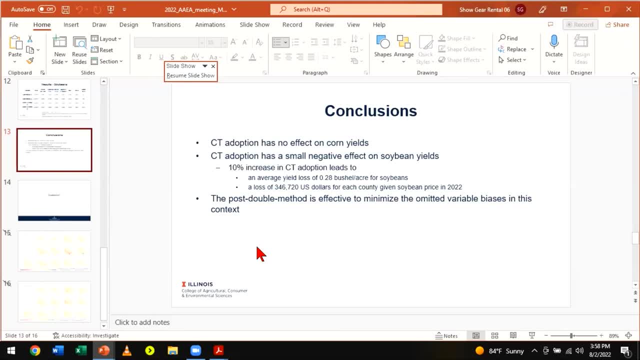 the expenses um from usba county level, us federal economic analysis analysis so you may change you the cost of the based product, of the product, the change of the cost of the expenses, I mean the input cost changes. Yeah, I use the difference of the input expenses. 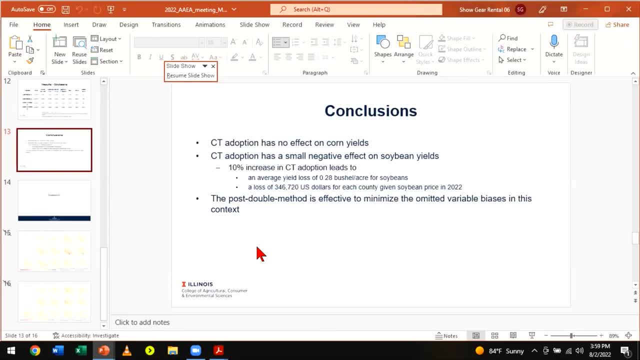 as one of the control to kind of predict the changes of the yield. For the incomes I use the lags, but for the expenses I think like it's highly related between the costs of the input and the yield. If you use more costs you may get a higher yield. 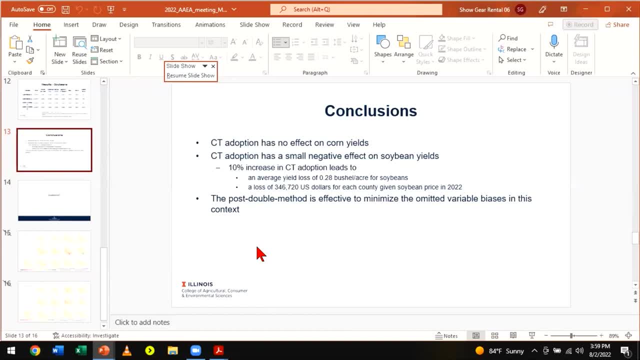 Yeah, I mean, I mean conservation may affect. I mean maybe you showed that conservation, Yeah, is going to affect operating costs. Yes, So the operating cost itself and think about the how long operating costs will change overall. 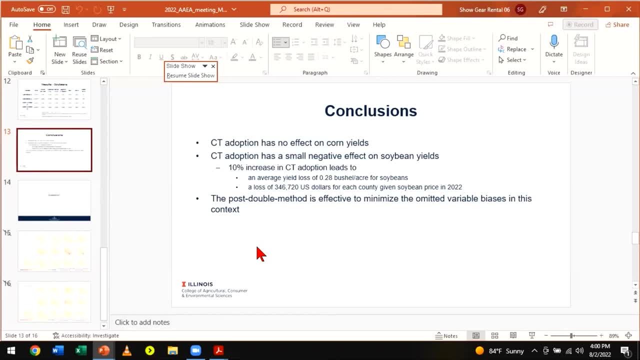 Yeah, Plus we have effect on yield. So then you can think about Yes, yes, yes, Thank you for your comments. I use like. I also use that like the differences of the cost use or the lag of the cost use. 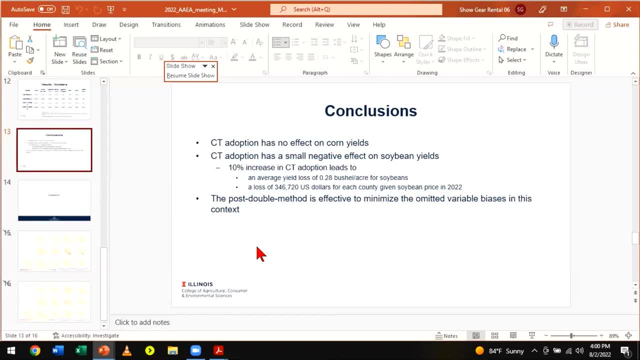 to predict the difference of the safety adoption. So pretty much after I go to the several variables that can predict the difference of the safety adoption, I kind of get a can the safety, the difference of safety adoption, taken as exogenous condition on all of those variables.